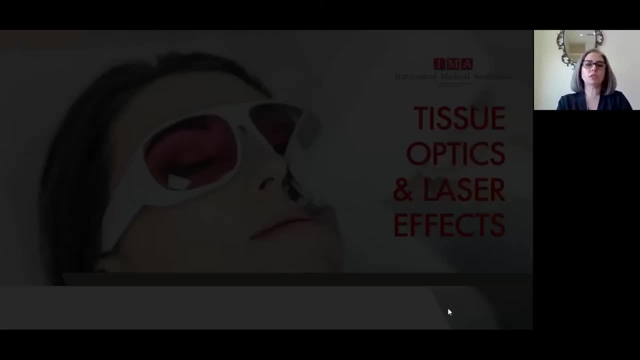 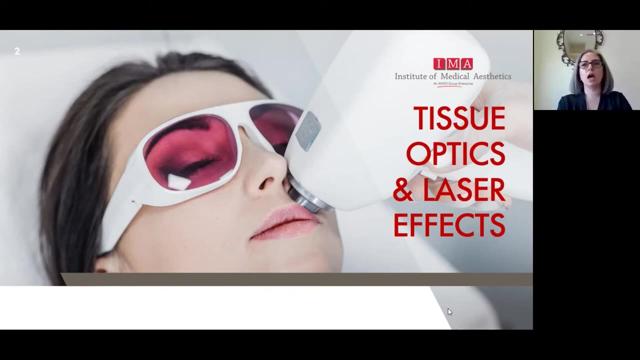 which is called tissue effects. Before going to tissue effects, tissue optics and what happens when I hit my skin with any laser, I have to have the basic information about laser physics. what is the characteristic of wavelength? what kind of wavelengths can I give to the skin? So these all come in different lectures Usually. 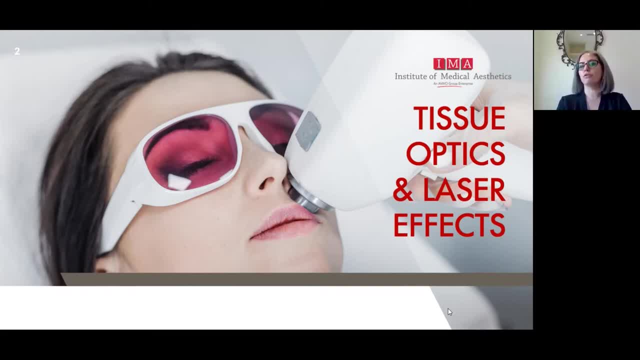 the first day of our course is a day full of lectures. We talk about several concepts that we want all the participants to pay attention to. And then we have the first day of our course, which is a day full of lectures. We talk about several concepts that we want all the participants to pay attention to. And then we have the first day of our course, which is a day full of lectures. We talk about several concepts that we want all the participants to pay attention to. And then we have the first day of our course, which is a day full of lectures. We talk about several concepts that we want all the participants to pay attention to. 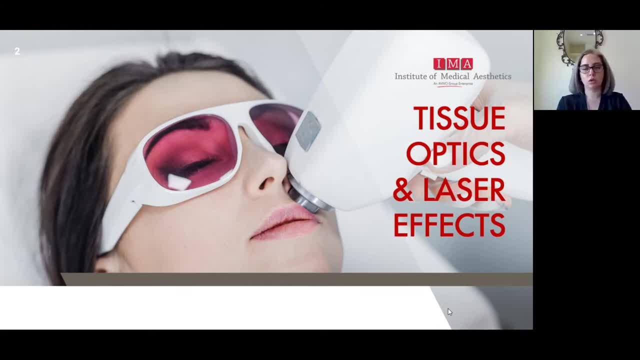 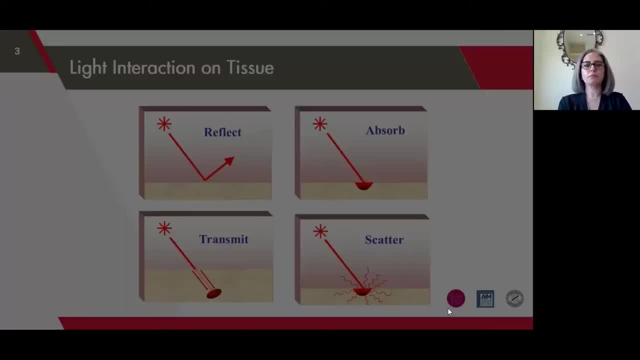 For every topic that we talk, we have the hands-on on the topic. This is just an example of one of the important topics of lasers. We know that We will start talking about it a little bit, Of course, before this lecture. 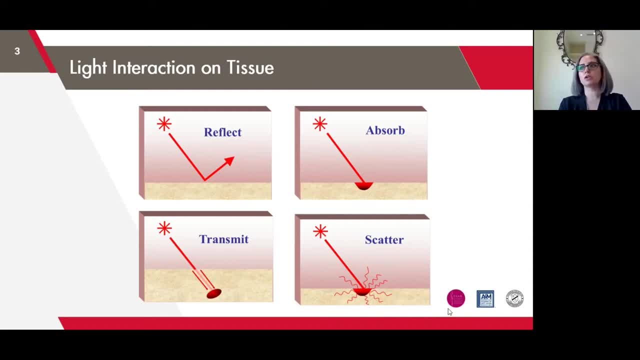 we talked already about the laser physics. We are supposed to know the characteristics of the light, the wavelength, different wavelengths with different skin types, classifications of the skin types. All of these we already finished with the lecture, Once we reach to this slide. 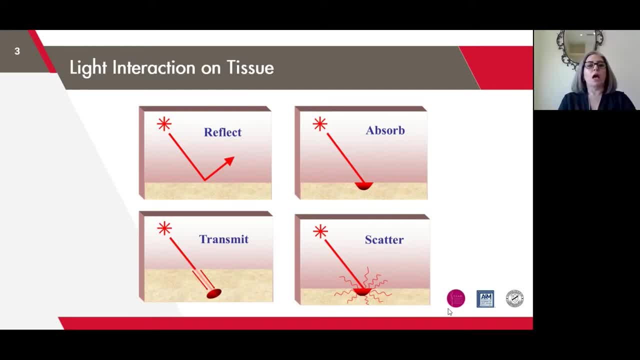 we are finished with the basic information Once we are here. this lecture tells us what happens to our skin when I hit my skin with any light or laser. The explanation is that, as you know, majority part of the laser gets absorbed by your target. I have means of controlling the other part. 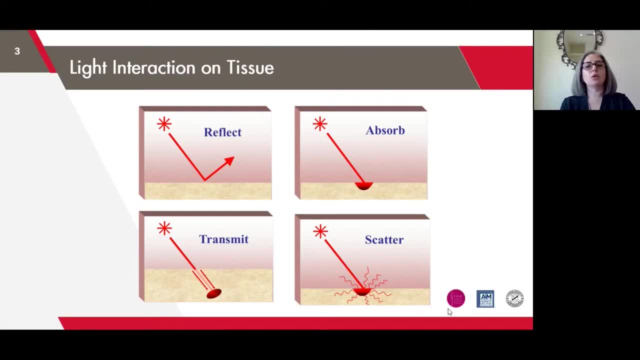 of the light, which is the scattered part. With the scattering, we always say: use a big spot size, because the smaller spot sizes they are much more prone to have a scattering effect. When talking about scattering, we always talk about using a high flux in laser, Of course. 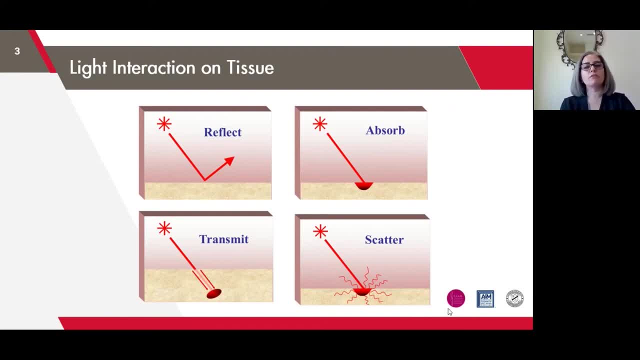 you have to know what is the meaning of high flux. When we are talking about high flux in aesthetics, we mean that using a laser in high power or shorter time Using a laser with a low flux will put your patient in a risk of skin necrosis because you are increasing the scattered amount of light. going to this, 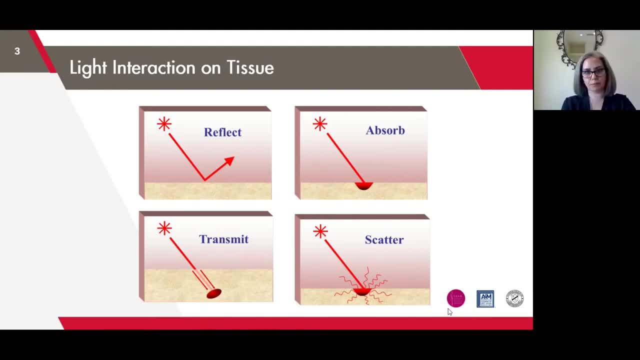 So so far we've talked about absorption and scattering. We have two other scenarios that might happen when I hit my skin with any laser. One is reflection. Fortunately, the reflection and transmission is neglectable part of the laser. You know that light's. 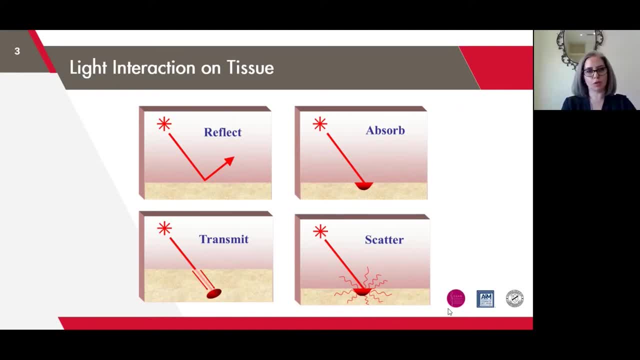 skin reflects more, dark skin absorbs more. it's like wearing white in the summer, wearing black in the winter. so lighter the skin i have, i have more, more reflection. that's one of the reasons explained to you why you don't have very good effect in hair removal in bony areas on your 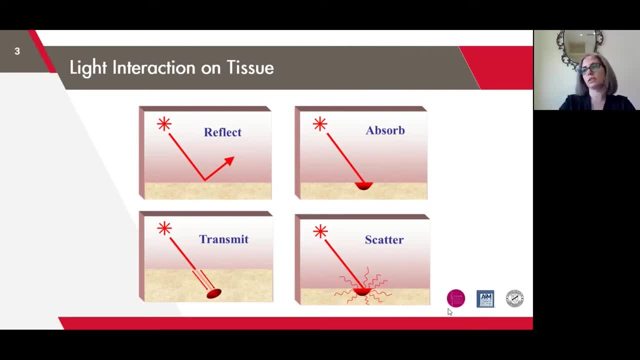 knees, on your fingers and your toes. why the result is not as good. now you know it's because of the bone underneath. because the white bone reflects so much of the laser backwards, the very, very neglectable part of the laser sometimes transmits beyond where i wanted to. 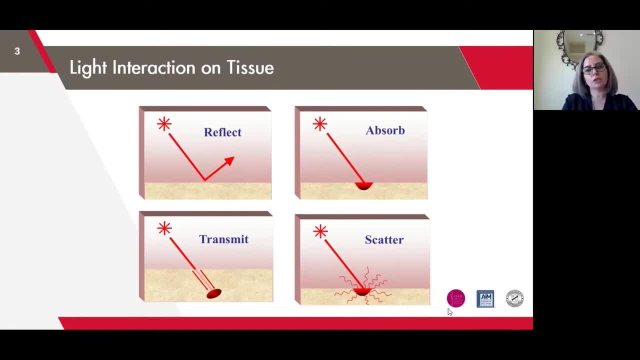 transmit, which now, with explanation, you should know that i don't have any means to control reflection or transmission. i cannot change the patient's skin type and transmission is not in my hand. so basically, with the parameters of laser, i am adjusting and arranging the absorption and scattering them out. this is a very, very important. 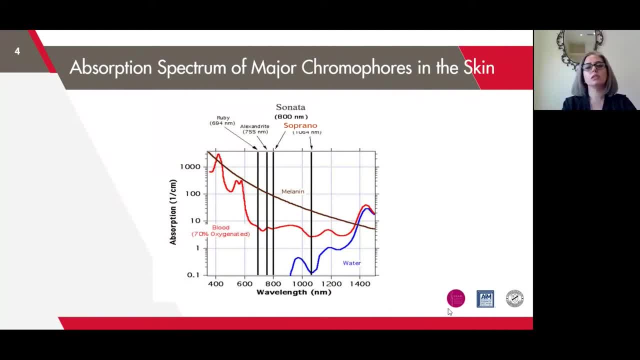 slide and basically what we do in aesthetic is all based on this slide. this slide tells you the absorption curve of our three chromosomes. the first and basic chromophore, primary chromophore of our body, is melanin. you know that we have melanin in our skin. we have melanin in our hair, we 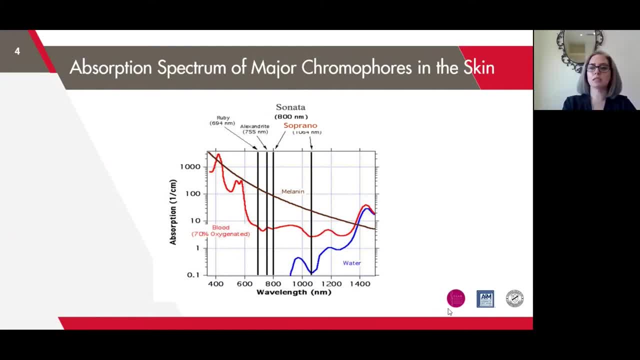 have melanin in our eyes. this is the pigment that we have and it's considered as our basic chroma. the explanation of this slide is the absorption curve of melanin, absorption curve of oxygenated hemoglobin, which is considered as our secondary chromophore, and the absorption curve of water. the term of chromophore comes from. 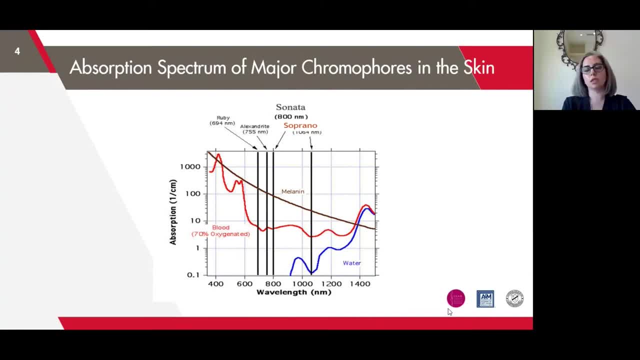 the greek term of chrome by the meaning of color, and four is anything that likes to absorb color. we call it chromophore. as we discussed, melanin is our primary chromophore, our secondary chromophore is oxygenated hemoglobin and our third chromophore, although 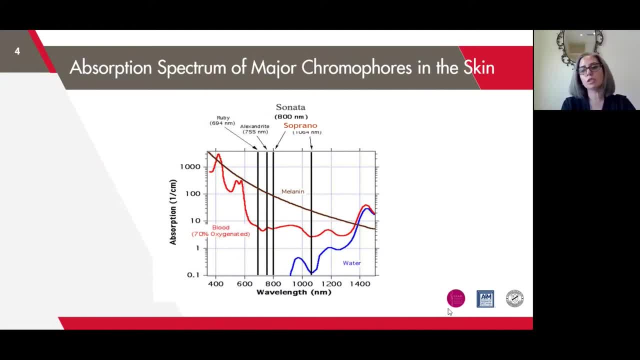 it doesn't have color but because it has absorption, is water. so, on this absorption curve, slide i will. i will see that melanin's absorption curve is a very easy, straightforward absorption. as you can see in melanin my absorption gets lower when i go in longer wavelengths. 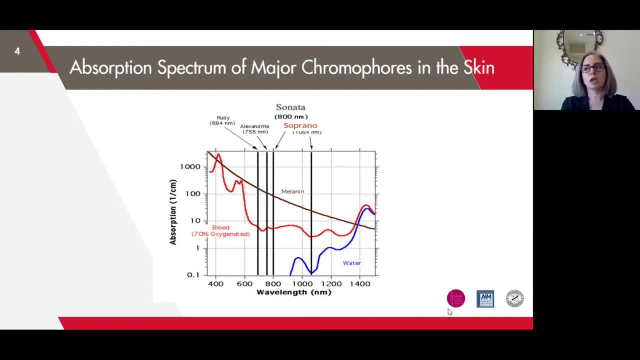 this means shorter the wavelength, higher the absorption in which treatments melanin is my chromophore, definitely in pigmentation treatments. in treating pigmentation, melanin is my chromophore, and in hair removal melanin is my chromophore for hair removal. you know that the first wavelength that we start treating the hair removal is 755. it's. 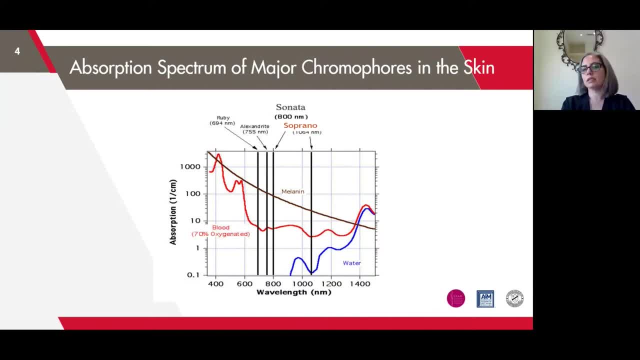 alexandrite. so some of you might think that why do i wait until 755 for laser to start? why don't i start with 400? because here the graph is showing me that 400 has much more absorption to 755. so why do i wait until 755 to start my hair removal? or sometimes 694, so for every treatment. 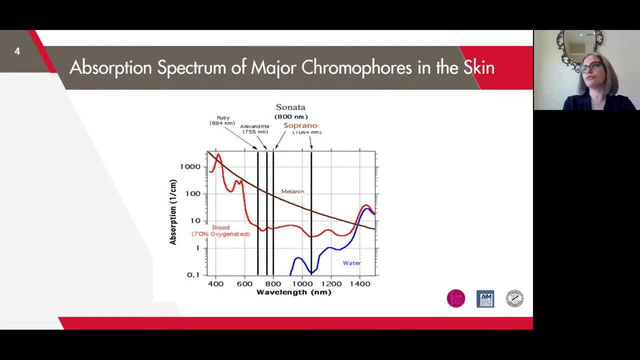 you have to consider two facts. one is the first is always the safety. safety tells me can i give a short wavelength to a dark skin time or not? this is safety. second one is efficacy. for efficacy, i have to define what is my target, and then where is my target located in the skin? 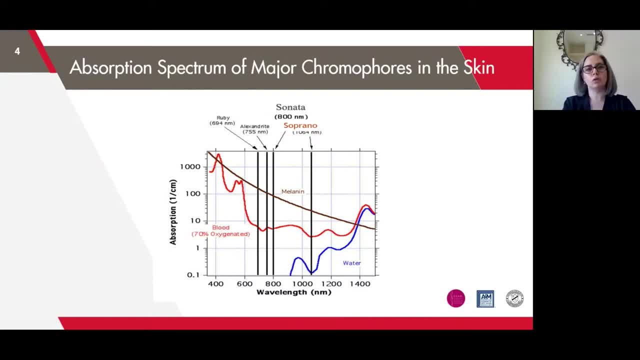 you know that when we are talking about hair removal we are talking about hair majority of our hair follicles they are in dermis, they are not in epidermis. when i have a shorter wavelength, according to our rule of electromagnetic spectrum, you know that shorter wavelengths they 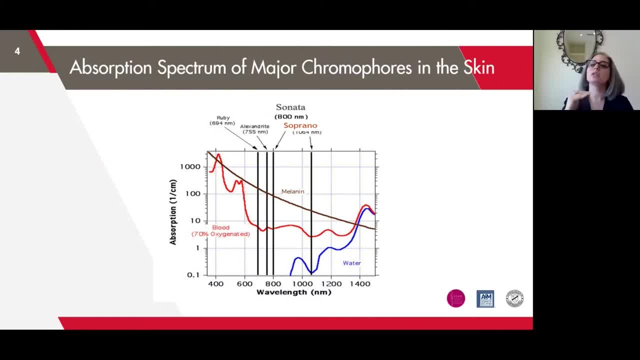 have higher frequencies but they penetrate very superficially. they cannot penetrate deep down in the skin. so i have to pick a wavelength that is able to reach to my hair follicle and then create a very long makeup to where my target is. that's why the first wavelength that we actually start 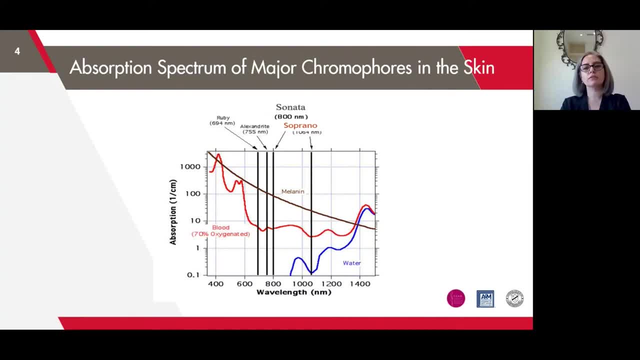 for hair removal is 755, and then longer wavelength after 755 will be a diet with 810 or 800 nanometer, and then the wavelength after for her removal would be india, 1064 nanometer, depending on the skin top. i have to pick what is appropriate for my skin type. 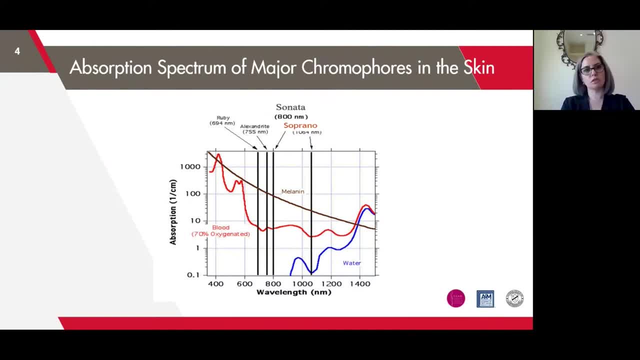 tells me never give an alexandrite to skin type 5. that's why i know that if i pick an mdiat my absorption is not as good as alex. but safety is my first rule. i have to commit to safety before committing to efficacy. this is about hearing. then my target is treating pigmentation. 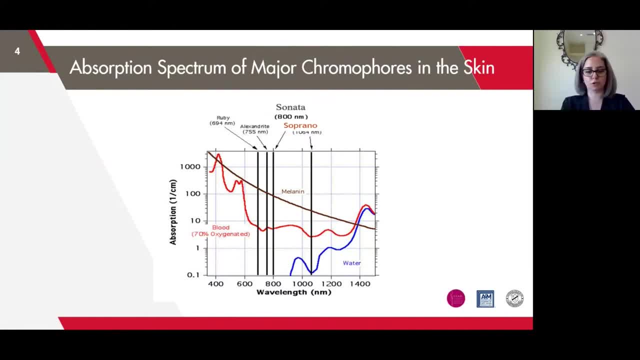 again, melanin is my absorption curve. we heard, or you have seen, or heard in aesthetics, that we say green is the best color for treating superficial pigmentation. then now, with this graph, you will know why: because green is the first wavelength that can reach to my epidermal pigmentation. 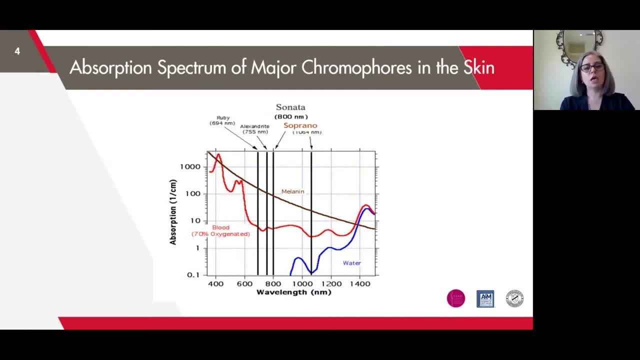 epidermal, not dermal. the second question again would be in: would the skin of melanin be able to treat superficial pigmentation? Which skin type can I give it green wavelength? Can I give it green to skin type five or even four? The answer is no. 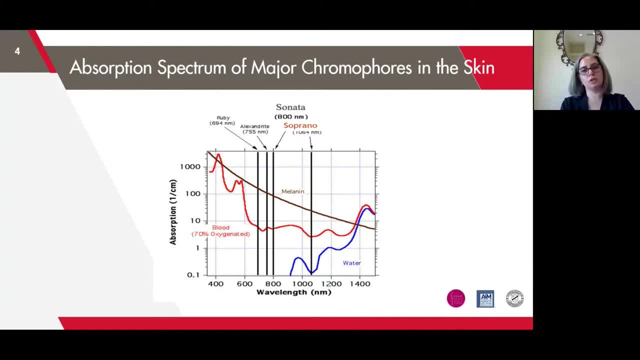 No matter how superficial is your pigmentation, you have to commit to safety first. So green is best color for superficial pigmentation if you have a skin type one, two, three, If your skin type is above three or your pigmentation is not a superficial. 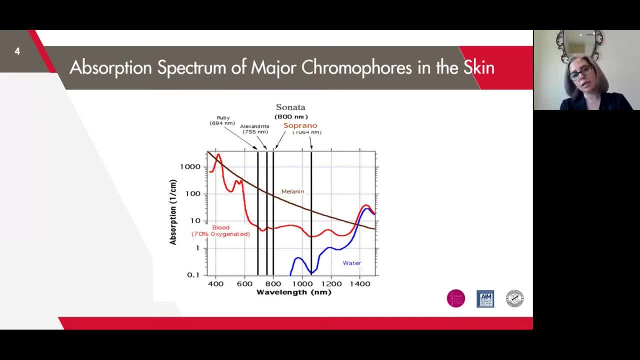 epidermal pigmentation is a bit of a dermal pigmentation, then you have no choice but to use a longer wavelength like NDR. This is when my melanin is my chromophore, Sometimes in some scenarios like telangiectasia. 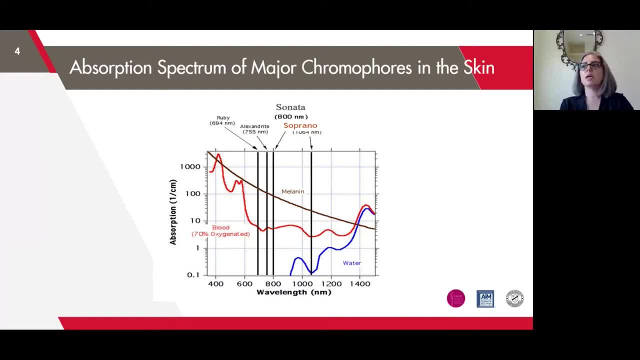 like chelangioma, like rosacea, my chromophore is oxygenated hemoglobin. As you can see in the slide, oxygenated hemoglobin again has a very good peak in 400. Which in practice is not practical because 400 doesn't penetrate in my skin. 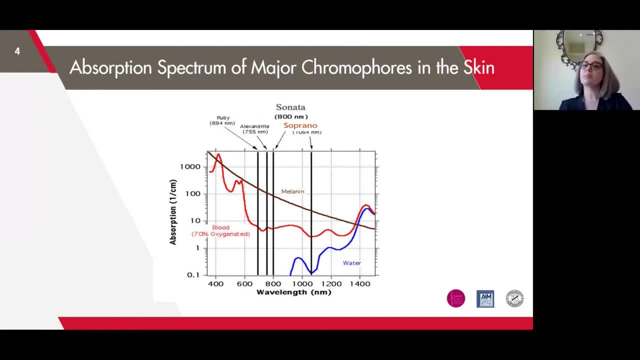 Even if I have a telangiectasia, it will be epidermal, It will be superficial telangiectasia, which I need to reach to it by a wavelength of the laser. So we say yellow is the best color for superficial red telangiectasia. 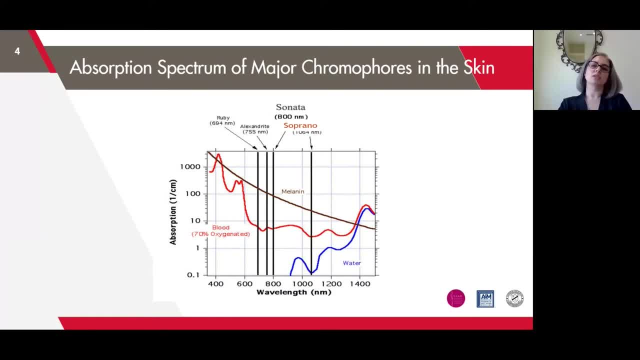 red vascular lesions, Because yellow is the first wavelength that can reach to my red vascular lesions are and it is in the peak of absorption. As you can see, the absorption comes down afterwards. Red on red doesn't have absorption. It means I can never remove a red lesion with a red laser. 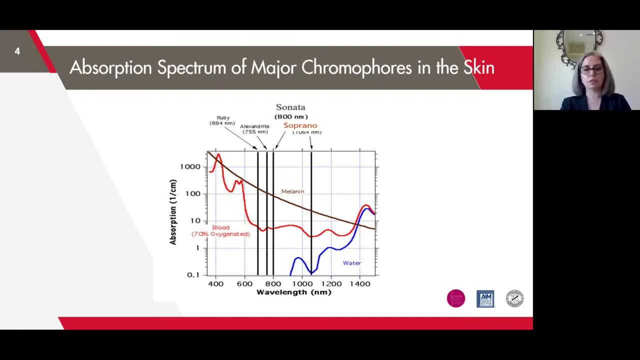 I should always target anything I want with opposite color of the laser. And then it continues a bit right until 1064.. So if I have again, my question would be: in which skin type would I give a yellow laser, regardless of how superficial and red the vascular lesions are? 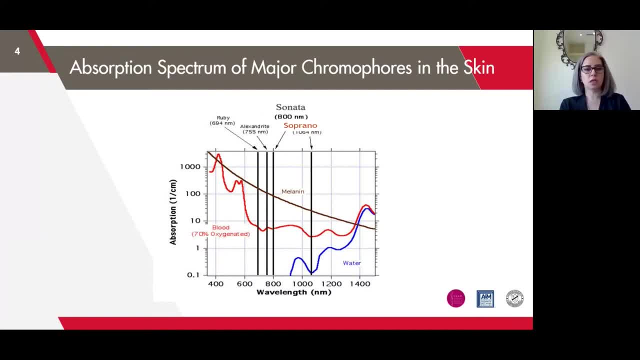 The answer again would be skin type one, two, three. This means if I had a skin type four with a red vascular lesion, or my vascular lesion was a bit deeper, it was a bit bluer and deeper, definitely you know that I'm not talking about varicose veins. 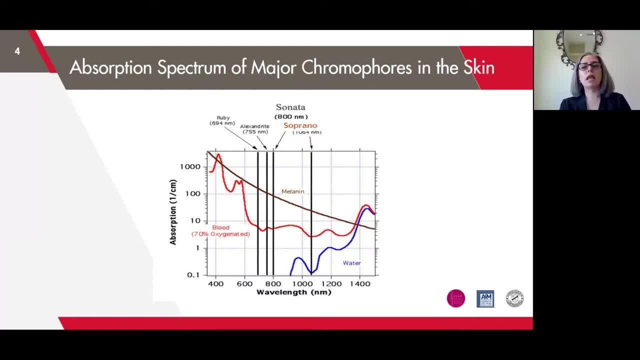 So if I had a deeper lesion or my skin type didn't allow me to use a yellow laser, then I have no choice again but to use an MDAG. So, as you can see, MDAG here in my aesthetic clinics is not only used for hair removal. 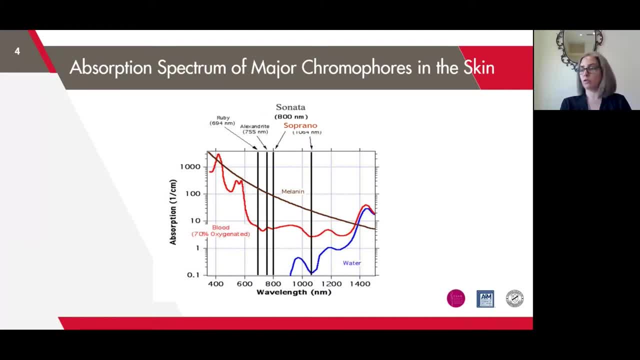 I can use it for my vascular lesion. I can use it for my pigmentation, depending on the MDAG. If I have a Q-switch laser, of course it's preferred to use it for pigmentation rather than the long pulse laser. 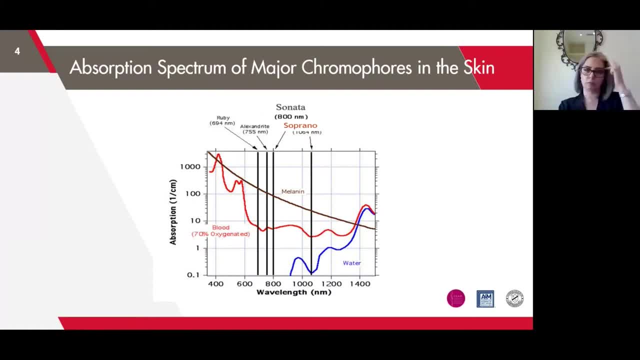 My third chromophore is water. You know that, Although it doesn't have color, but it absorbs the laser. That's why, for me, it's considered a chromophore. So water absorption. as you can see before the number, 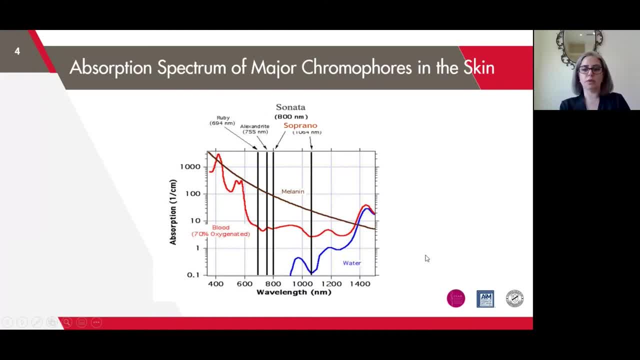 we have a very important number in laser, which is 1,400.. Water absorption: before this number is neglected, I don't consider water absorbing anything before this number. Water absorption: before this number is neglected: I don't consider water absorbing anything before this number. 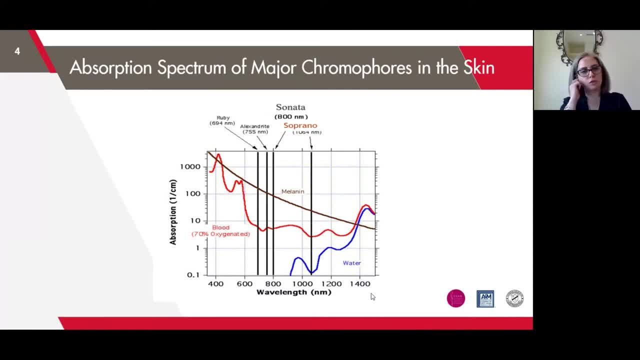 Water absorption for me starts from 1,400.. I want you to remember a point: that the more water absorption I have, the more superficial I have a laser It is. You know that we are contained in water. 70% of our body weight is water. 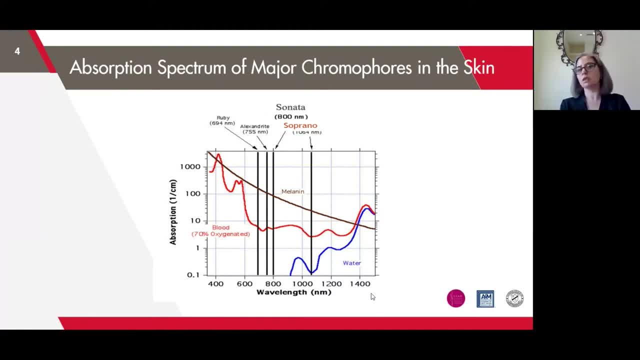 So where do we have water? All the cells in our body, including our epidermal cells. So when I'm giving a laser, that it's after the water absorption, after the range of water absorption. the best peak of absorption is at the range of Airbnb, which is 2940.. 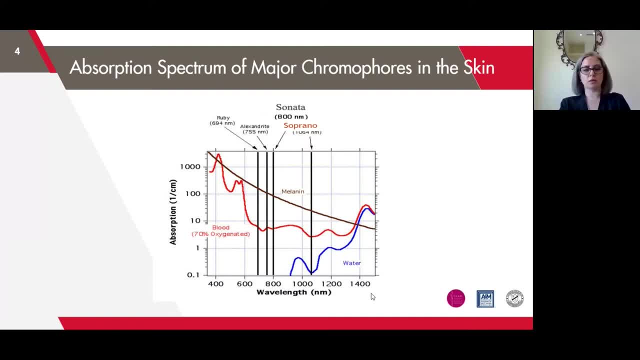 And then I have the second peak at CO2, which is 10,600.. So when I have the peak of water absorption, whatever laser I give, it's absorbed by the first line of epidermal cell. The laser is used all in order to water absorption. 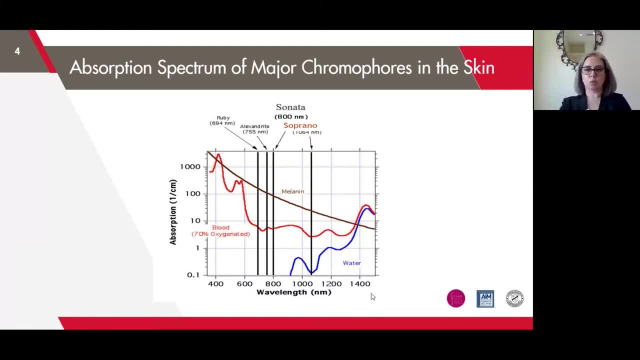 When the laser is used and absorbed by water, the heat of the laser goes beyond even 70 degrees, goes above 100 degrees and starts boiling and evaporating the water. By evaporating the water, it evaporates the cell and tissue that was within. 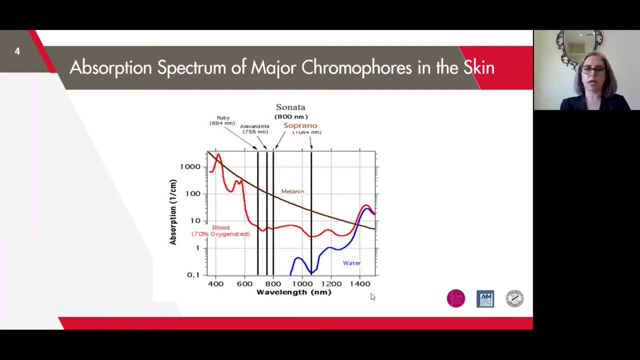 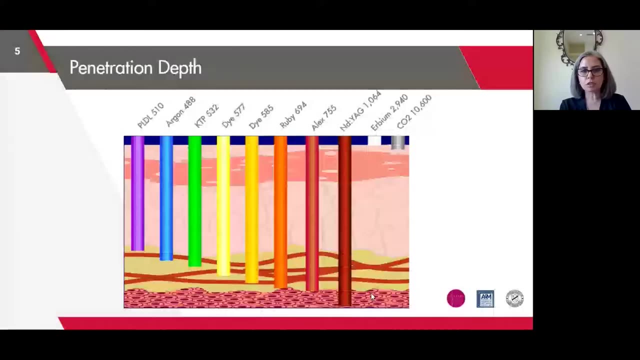 The water was within. So that's how Airbnb preserves or ablates the skin by boiling the water. So I want you guys to remember: the more water absorption, the more superficial your laser goes. As you can see, this is just a schematic view to show you that longer the wavelength 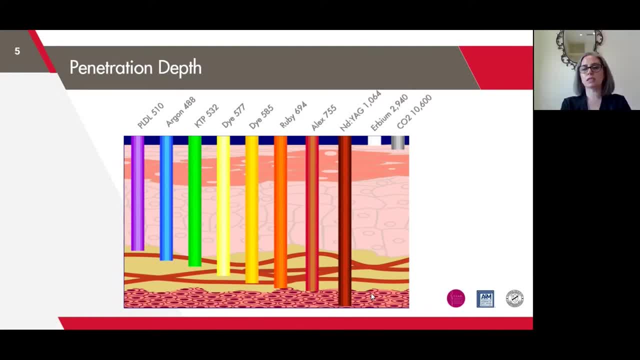 deeper the penetration And once you have the Airbnb and CO2 that they are after the range of absorption. actually they are the two peaks of water absorption. I want you to pay attention how superficial your laser is. Again, the same concept, approximately. 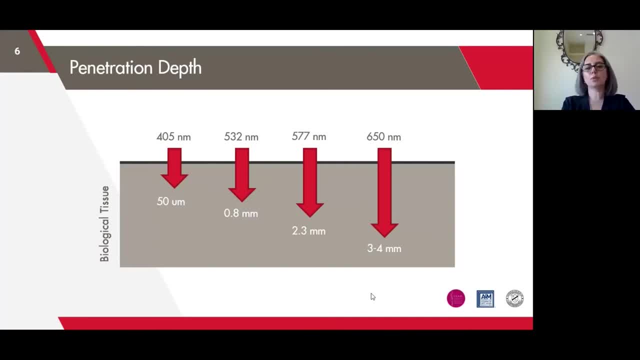 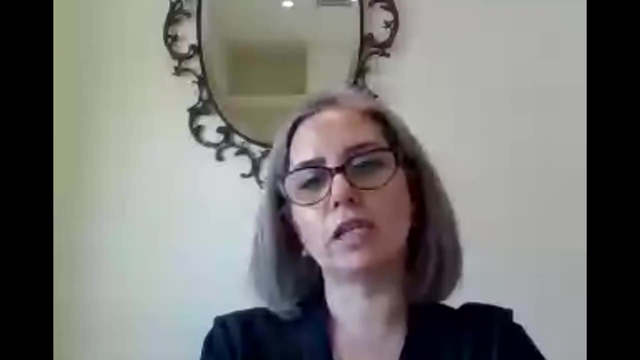 With a blue laser, I have 50 microns penetration depth. With a green laser, I have less than one millimeter. With a yellow laser, I have approximately two millimeters. With 755, I have approximately three millimeters penetration depth. 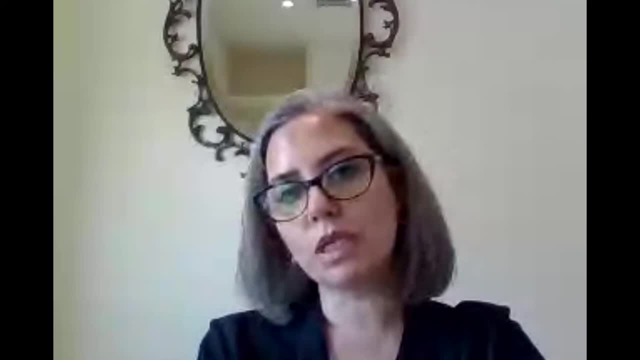 And with NDF I have approximately four millimeters penetration depth. The mechanism that I work with, usually with long pulse lasers, as you know, it's heat. I work with the mechanism of heat. It means I give a laser, absorb this laser absorb this light, the light transferring. 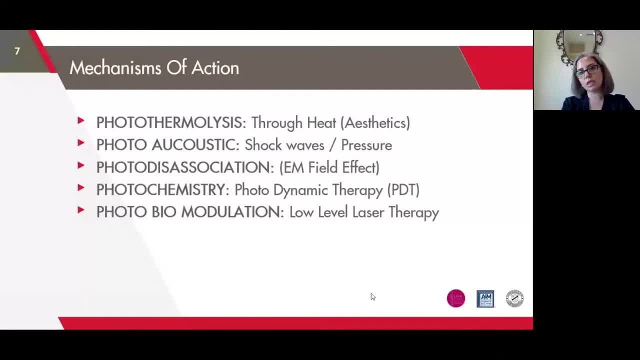 to heat and I want the heat to be to the extent of killing or lysing or cooking my target. This mechanism is called photothermal lysis. It means I gave a photo which is my laser. this photo turned to thermal effect. this thermal was to the extent of lysing, my target, and I have 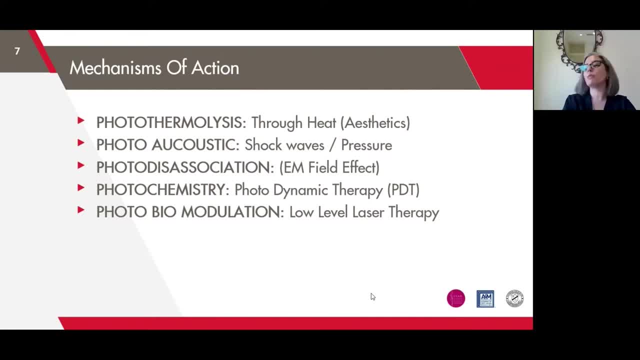 to be careful to do it selectively. That's why, majority of the times, the mechanism of majority of what we do is a selective photothermal lysis. Photoacoustic is the mechanism of Q-switch lasers. Q-switch lasers, they are fast lasers, The difference between a Q-switch and a normal. 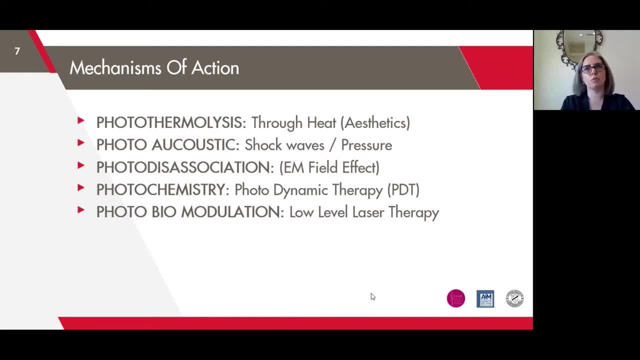 laser. you know that for all the wavelengths I have the Q-switch format, I have Ruby, I have Q-switch Ruby, I have Alex, I have Q-switch Alex, I have NTF, I have Q-switch NTF. The normal lasers that we can do selective photothermal lysis are referred as LP. 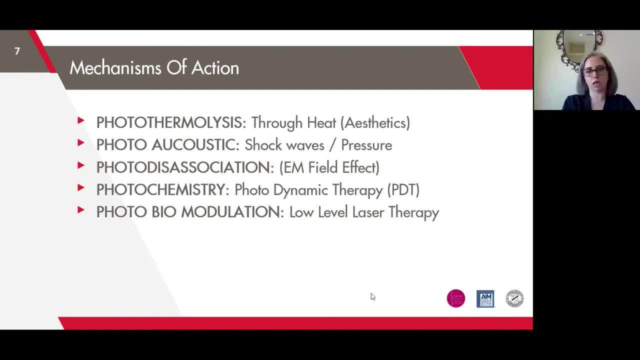 long pulse lasers. So you will find LPI, LP, Alex. This means it works with a mechanism of long pulse. Long pulse lasers, their pulse duration: pulse duration: it's the time it takes for the laser to come out of the handpiece With long pulse lasers. 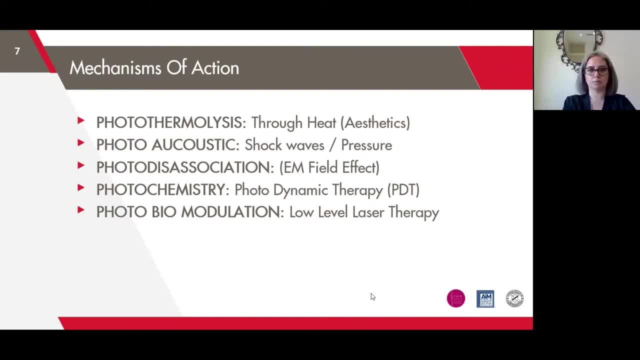 your pulse durations are in milliseconds. With Q-switch lasers, your pulse duration it's in nanoseconds. So now that you have such a fast laser, remember that Q-switch laser doesn't have time to create this heat. There is no time to reach to 70 degree and 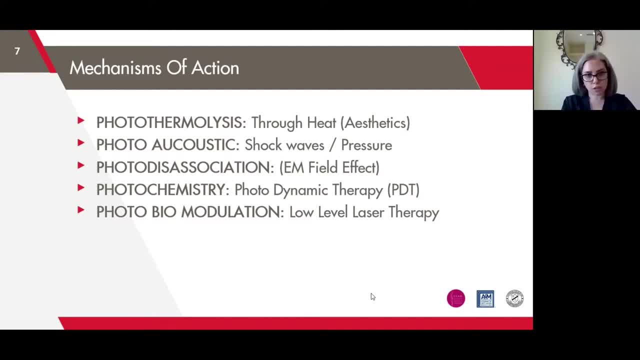 kill my target with heat. Photoacoustic lasers or Q-switch lasers: they basically shiver, create a cold pulse. They also have the ability to allow light to escape through. OctoBot Acoustic mechanism is a mechanism I use for tattoo removal. I cannot heat up the tattoo. Tattoo is. 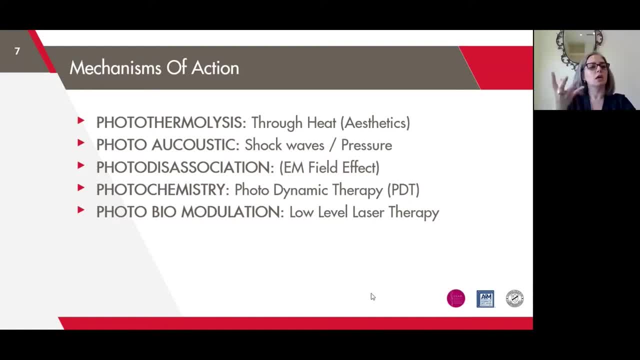 a color part. it absorbs my laser. it burns the skin, blister and burn and turns to third degree. So over the tattoo, I have no choice but to use something that doesn't heat up the ink of the tattoo. I'll come and shiver and basically burst. It's a little bit like the光 that I use in an 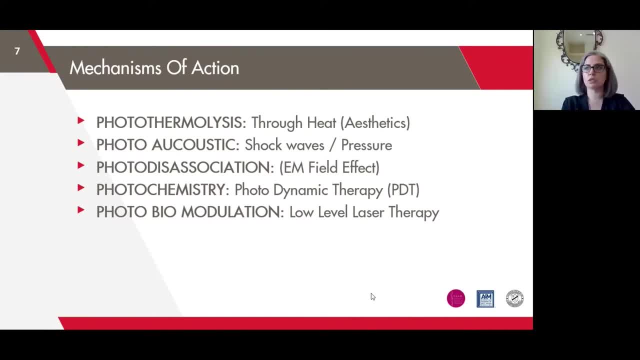 the tattoo ink with smaller particles until my body comes and photosites the tattoo, the small inks. what else am i using it? nowadays i'm using the q switch lasers in pigmentation. you know that melanocytes and heat- they don't work good together. they are not good friends with each. 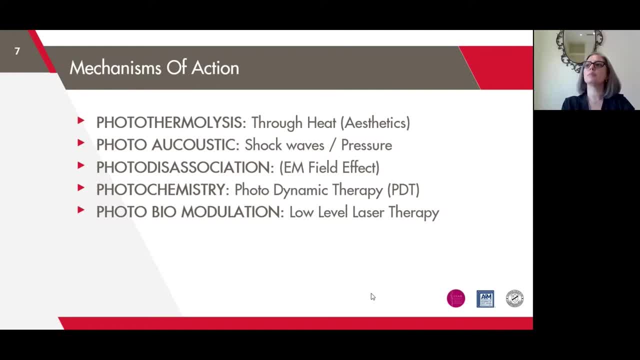 other. you know that melanocytes- anytime you give them any heat, even during this hot summer days, melanocytes can get stimulated and give you more pigmentation, more problems. so anytime i am suspecting a patient to be pigmenty problem like melasma, the lentigo, generally pigmentation, pih- i always prefer to target it with a q-switch laser than in. 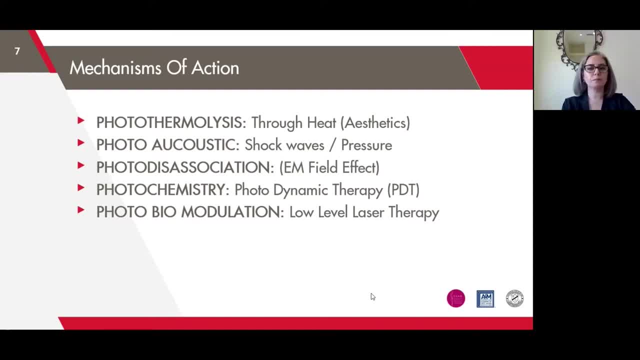 long pulse laser because it has less heat. photo disassociation is the mechanism used in ophthalmology photo. so chemistry is used in uh photodynamic therapy. you know that photodynamic therapy started from cancer lesions. they give a photosensitizing medication to the patient and definitely in. 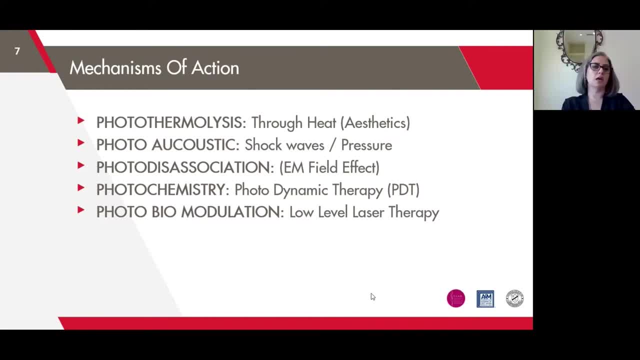 the tumor which i have, the accumulation of cells. i have more absorption of this, more photosensitizing medication, and then i shoot this area with the lights that it's sensitive to, with the laser that this tumor is sensitive to, the light. photodynamic therapy is a starting. 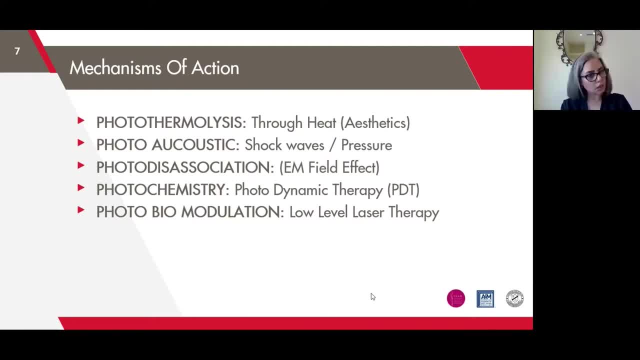 to come in aesthetics as well. it is still not in practice, so much so, but it's starting to be practical in aesthetic as well. photobiomodulation is the mechanism used in leds and when you go to spa and they hold the light with distance from your skin. five minutes, ten minutes. 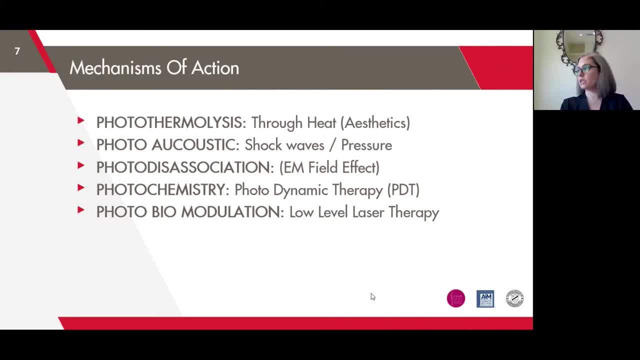 blue light, red light, yellow light. definitely, you have to know that with these low level laser therapies, leds are referred, referred as lllt's low level laser therapists. definitely i have to know that when i'm holding an led, i cannot expect under my skin to reach to 70 degrees. how do i expect? 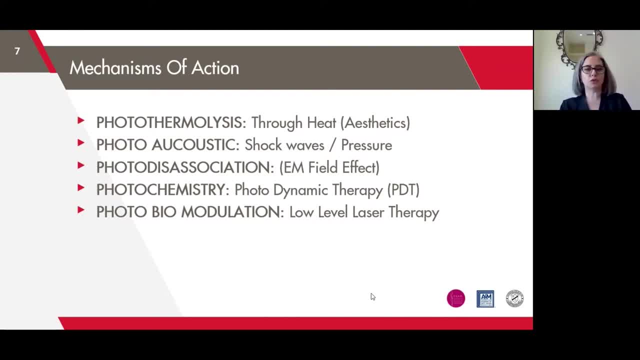 that leds they do some kind of rejuvenation, because they do a bit of a determination. it's not as strong as my class for lasers that they do thermal lysis, but of course they do rejuvenation. so how do they do that? You know that our breathing organelles, the ones that define the metabolism of the cells, are our mitochondria. 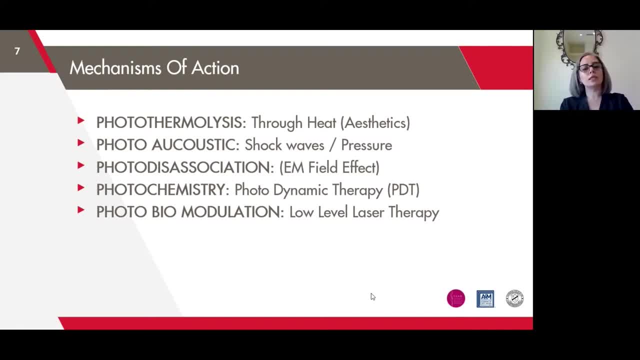 We know that with LEDs, with low-level laser therapies, mitochondrial activity in enzyme production in metabolism increases. So basically they biomodulate mitochondrial activity and enzyme levels. That's why the rejuvenation you get it's minor rejuvenation. 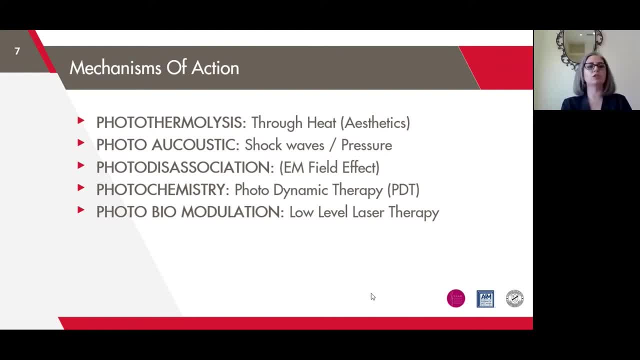 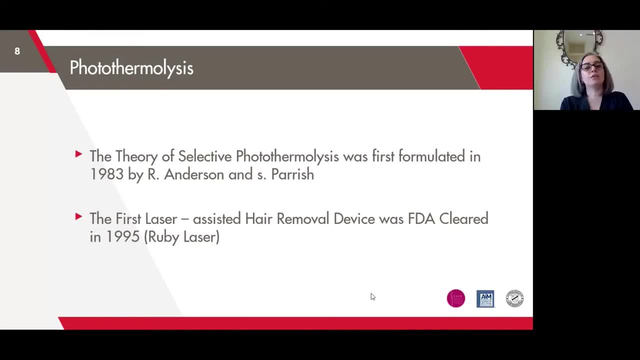 You see some difference, you see some rejuvenation, you see improvement, but it's not as much as a class 4 heat treatment. The first time that the theory of selective photothermalysis was discussed was in 1983 by Rox Anderson and Parrish. 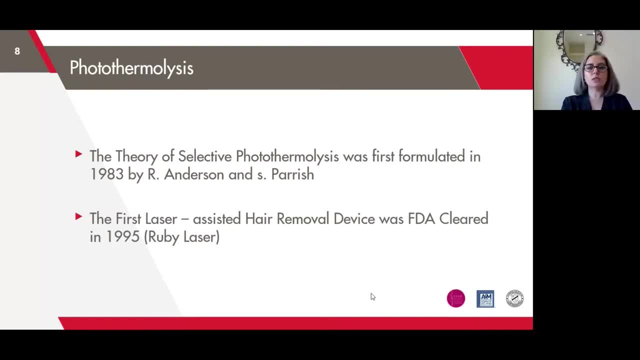 The first time that the first laser was made was 1960 by Theodore Maiman, Which was a ruby laser, and maybe it's interesting for you that it was 1960 that the first laser was made. But it took 35 years for FDL to clear this laser as a permanent hair reduction. 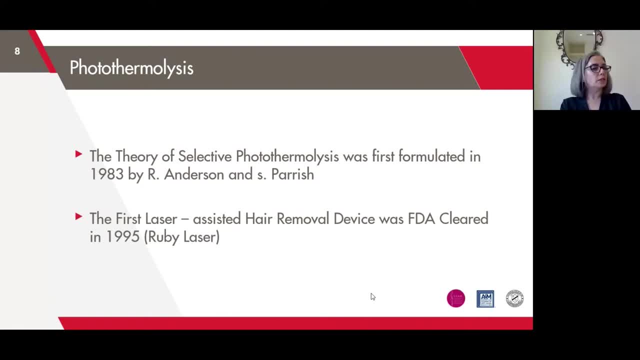 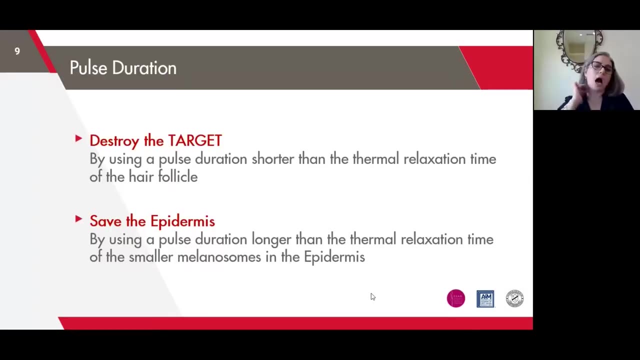 And for some of you who didn't know this information, IPLs came 30 years later than lasers in the market. The first laser was 1960, the first IPLs- they came in 90s. So how can I make sure? what is the selective photothermalysis? as I told you, 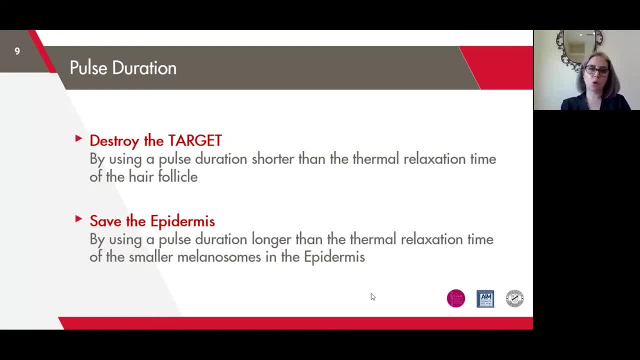 In theory of selective photothermalysis, I'm talking about destroying my target without destroying the surrounding tissue, not even the epidermis. So how can I do that? By a concept named thermal relaxation time. You know that to any structure, when I give heat, 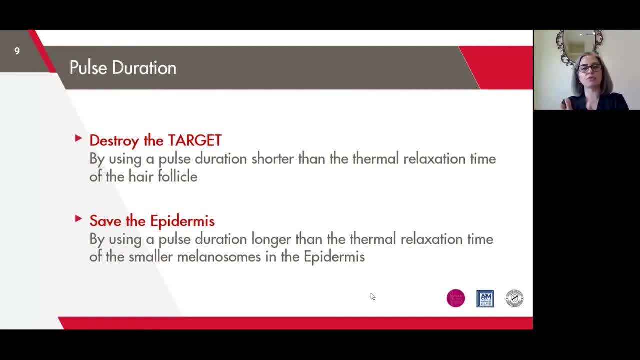 the time it takes for half of this heat, or 50 percent of the heat, to be dissipated. this time is called thermal relaxation time. Thermal relaxation time is the time that depends on the size of my structure. It means smaller structures. they heat up faster. they lose the heat faster. 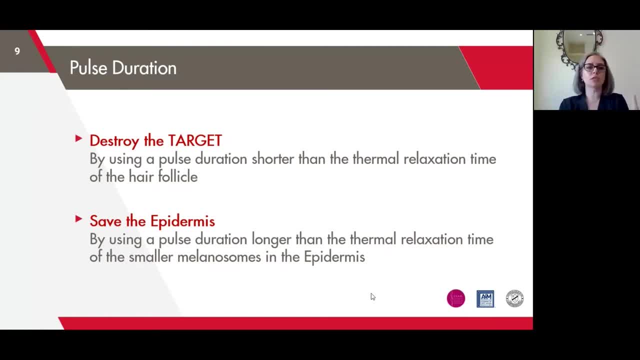 It's like when I want to drink a tea and I want to boil this much water, or when I want to cook and I want to eat, to boil this much water. definitely this much water boils faster and if i don't drink my tea in five, 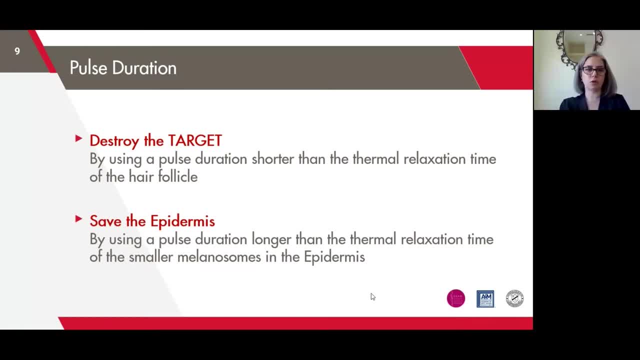 minutes. it's cold, but this much water holds the heat for longer time. so smaller structures. they have quarter thermal relaxation time. when you want to do any aesthetic treatment you have to have the thermal relaxation time of two structures. one important one is epidermis, because your aim is 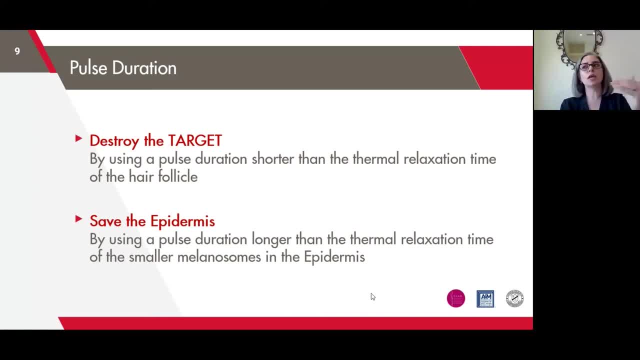 never burning the epidermis and your aim is destroying your target. whatever your target is, for example, if you are doing hair removal, you have to know the thermal relaxation time of your hair epidermis and you have to know the thermal relaxation time of your hair follicle. yes, so in. 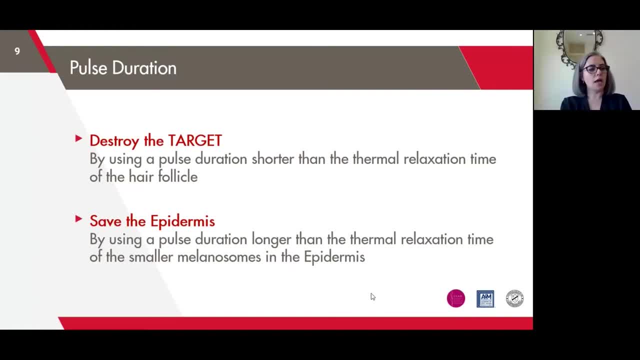 order to have a successful hair removal, i have to save the epidermis. i should never save the hair follicle. i have to kill this. i have to save this. how can i save epidermis? i have to give my laser in a way that my epidermis has time to cool down. it means my whole duration of the laser will be. 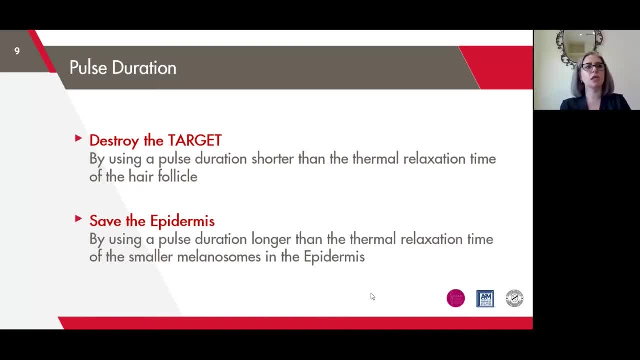 longer than the thermal relaxation time of the epidermis, because my aim is to give a chance for epidermis to cool down, but when my aim is not to give the chance to my hair follicle, my pulse duration should be shorter than the thermal relaxation. 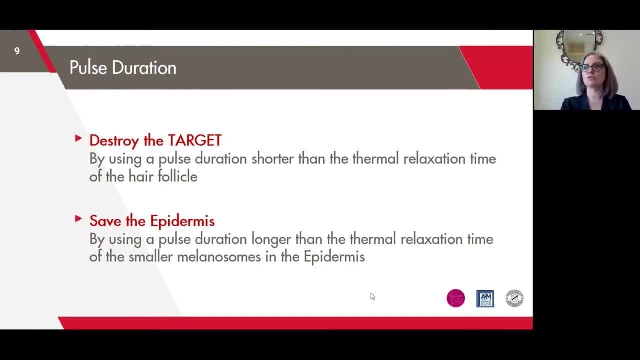 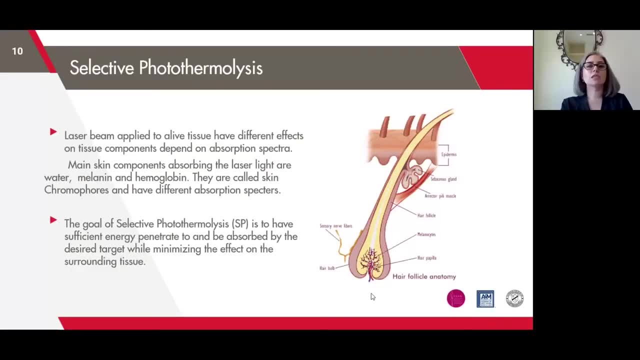 time of my hair follicle. in this way, i can guarantee that i saved epidermis. i didn't save hair follicle. that's why thermal relaxation time is a very, very important concept. so selective photothermalises. it tells you that to give the laser, your target absorbs the laser, depending on 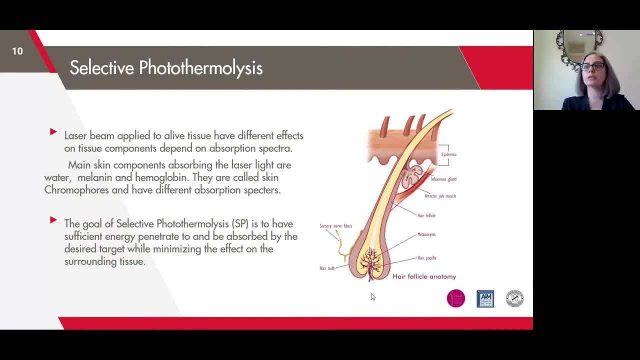 the chromophore. as we discussed, our main chromophores are melanin, oxygenated hemoglobin and then water, depending on the chromophore. your chromophore absorbs the laser gets heated, gets cooked, killed light without you damaging the surrounding tissue. this is called selective. 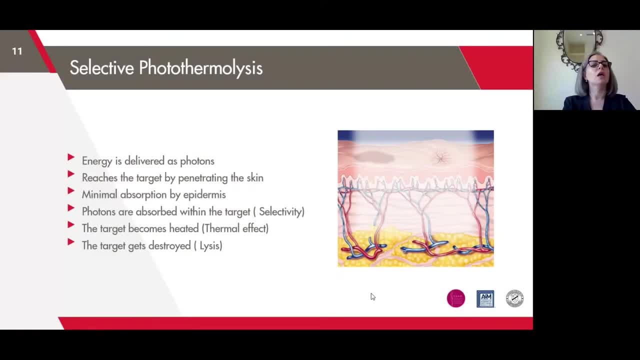 photothermalises, energy is delivered as photons reaches the target of the hair follicle and the laser reaches the target by penetrating the skin. minimal absorption by epidermis. how can i make sure that my epidermis doesn't get hot? guys, i want you to pay attention that there is no hair removal. 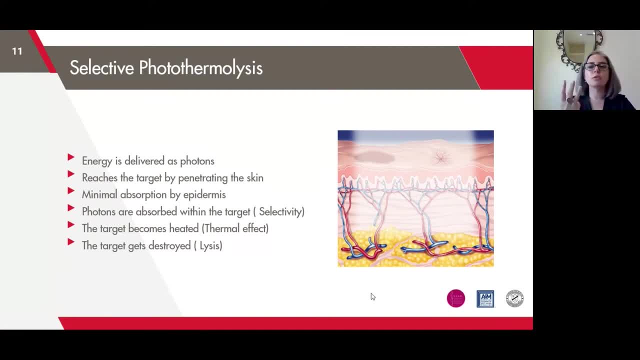 without a cooling, and by cooling i mean only three methods of efficient cooling. the most efficient, the most effective cooling is called cryogen, which is referred as bcd dynamic cooling device. the second best cooling is contact cooling, which your handpiece has a sapphire inside of it and 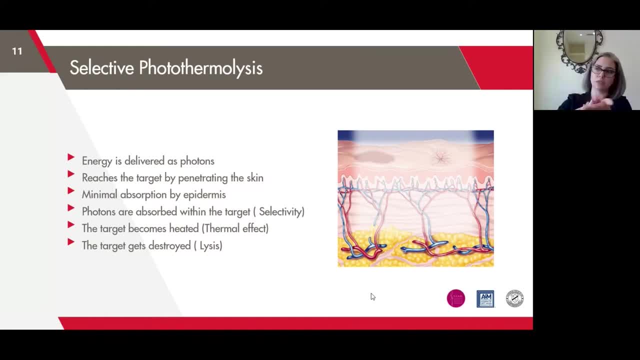 water circulates around keeps the surface of your handpiece cold all the time. if your handpiece didn't have a contact cooling or you don't have cryogen placed in your device, then you have to bring a zimmer as a cooling method. please pay attention that gels and ices are not considered. 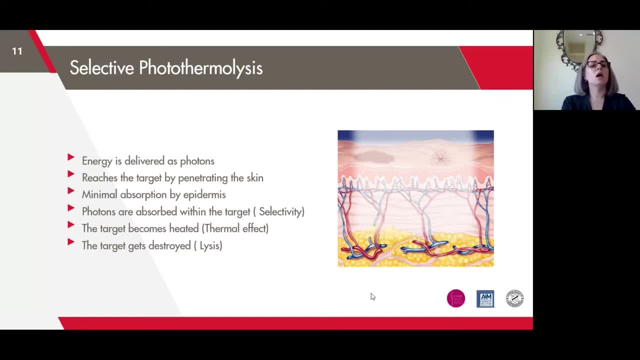 efficient cooling for me. so minimal absorption by epidermis. photons are absorbed within the target. my target absorbs the laser more than the rest of the tissue. the target becomes heated. this is the thermal effect and the heat is to the extent of dicing my target, cooking or killing my target. this is a 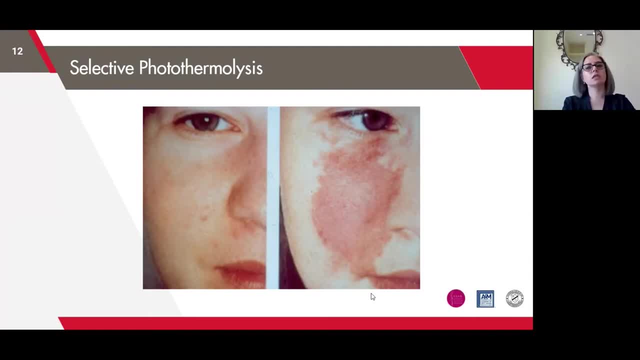 photo showing you an example of a selective photothermalises. i just removed the lesion without removing or burning or damaging the photothermal lysis, and this is the photothermalise surrounding tissue. So, as we said, thermal relaxation time is the concept that I can. 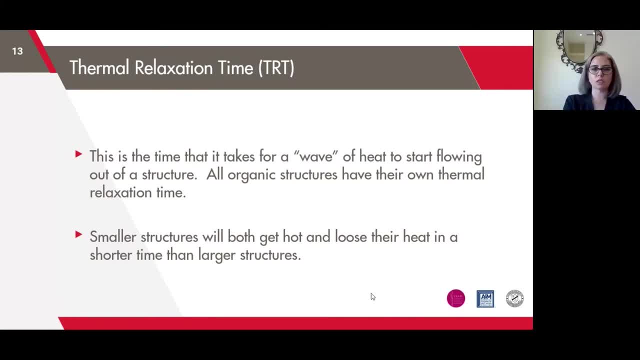 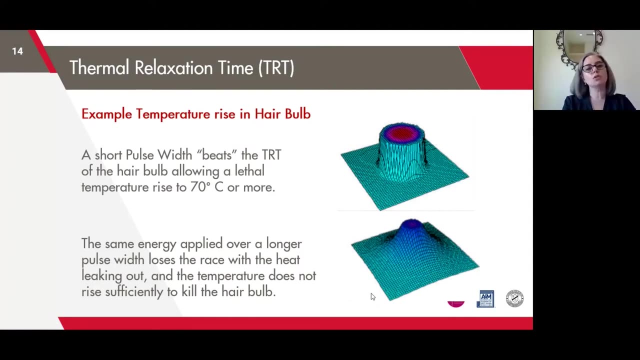 guarantee I do selective photodermalysis without damaging the surrounding tissue, when I know what is the time I have to give to which structure. So when I'm giving the pulse duration in a short time, I'm basically not letting the heat go away. 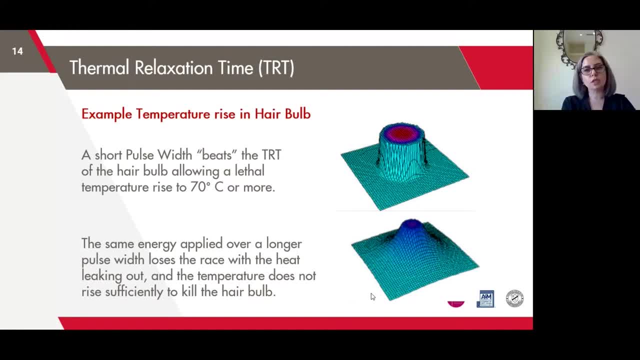 Okay, That's why my short pulse duration works when I want to aim carefully the gall or anything of the sort. If I give a pulsed duration in a long time, I'm basically giving the chance for the structure to cool down. So always my thermal relaxation time is longer than my. 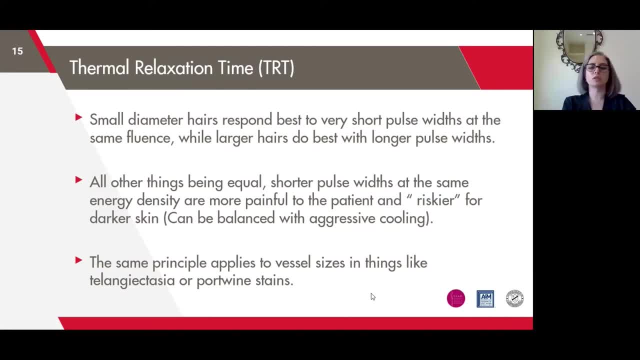 epidermis shorter than my target. whatever is my target? If it's hair follicle, my target is hair follicle. If it's blood vessels, I have to know the thermal relaxation time of blood vessels. Of course, the shorter pulse durations. it's more zappy, more uncomfortable. 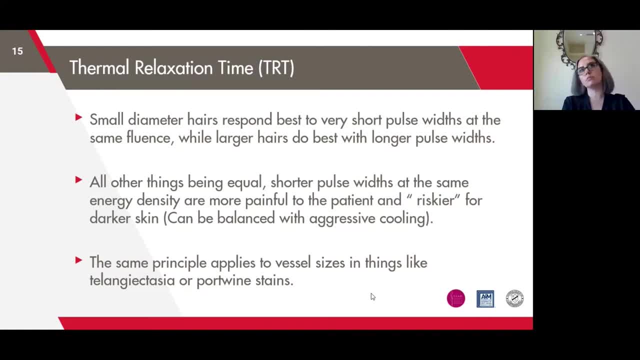 more painful And I have to consider that sometimes I can never give a short pulse duration. which is who? Dark skin types? Dark skin types, they cannot take a short pulse duration. Please remember, pay attention, that giving a laser in a short pulse duration is 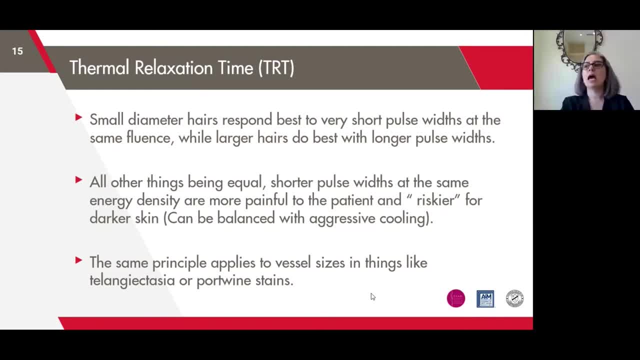 like emptying the bucket of water all at once. And when I have a dark skin my skin cannot take it. So with a dark skin, I don't need to give a short pulse duration. I can give a short pulse duration. I can give a short pulse duration. I can give a short pulse duration. 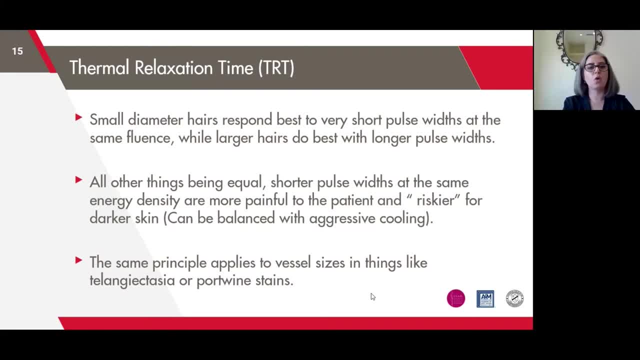 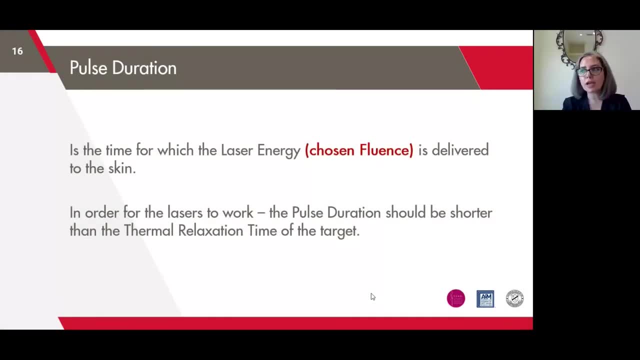 I need to look at the hair color. I always consider the skin color, But when I have a light skin, in that scenario I can check and look at the hair color. When my hair is terminal, thick, dark black-rooted, it means the thermal relaxation time is longer When 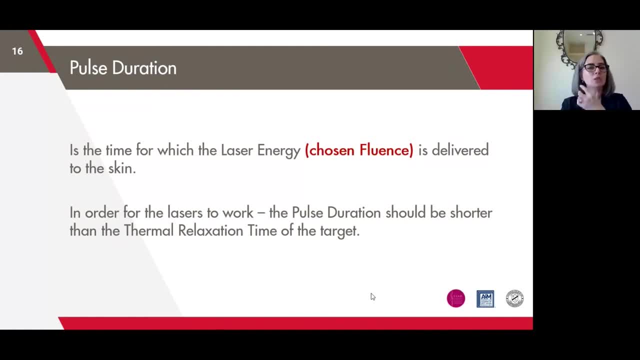 I have a light peach plus hair. blond hair in my face means the thermal relaxation time is shorter than my target, So I have to attack it with a shorter pulse duration. Lighter the hair needs shorter pulse duration Only in scenario that my skin type allows me to do the short pulse duration. 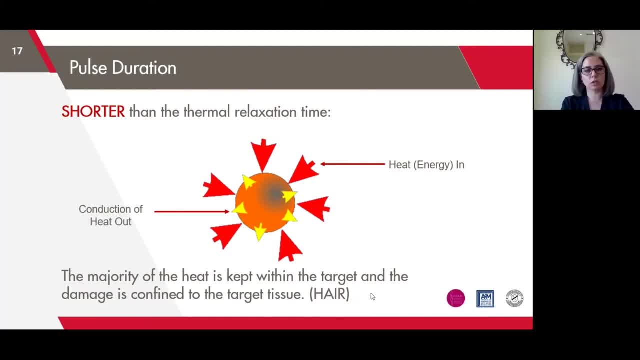 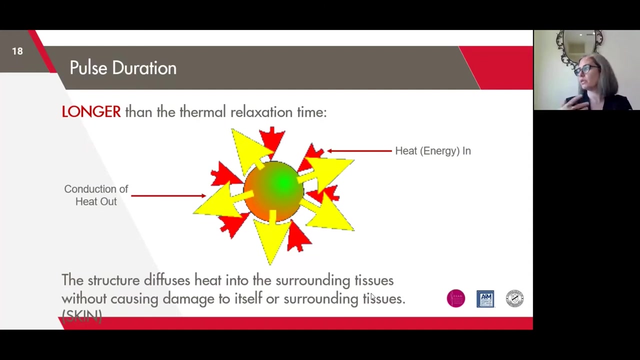 So these are all important concepts that I want you to be aware of them. When you are giving the heat shorter than the thermal relaxation time, you are keeping the heat inside and your aim is healing. When you are giving the heat longer than the thermal relaxation time, you are basically giving the chance for the structure to cool down. 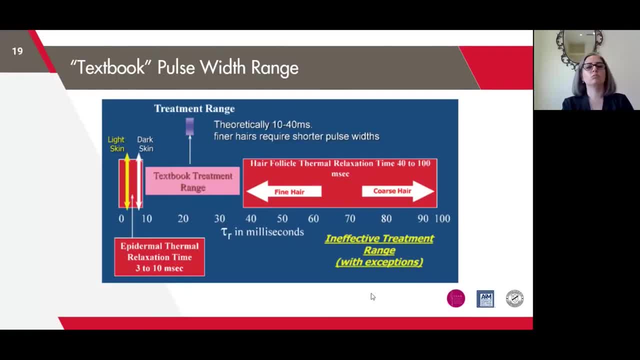 Your aim is saving. Here is the two important structures you have to know: In epidermis, my thermal relaxation Time is 3 to 10 milliseconds. in my hair follicles, My thermal relaxation time is 40 to 100.. My hair in my face, if it's light, it's approximately 40, 50 that. my hair in my armpits, maybe bikini, or my scalp or men's beard. 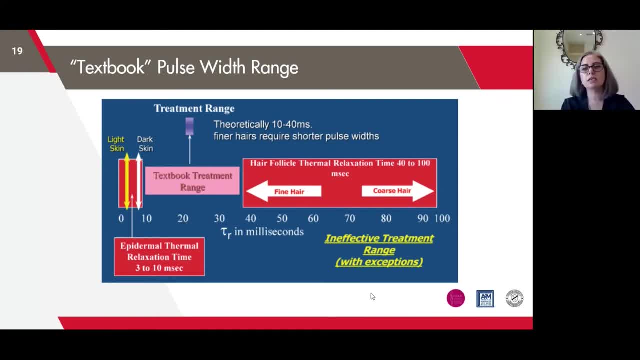 Or when I have a dark hair, that hair's thermal relaxation time is 100. Or near to 100, depending on the color of the hair. That's why you always ask your patient: what is the color of your hair, As we discussed, if my skin type allows me- like me, I am skin type 3.. 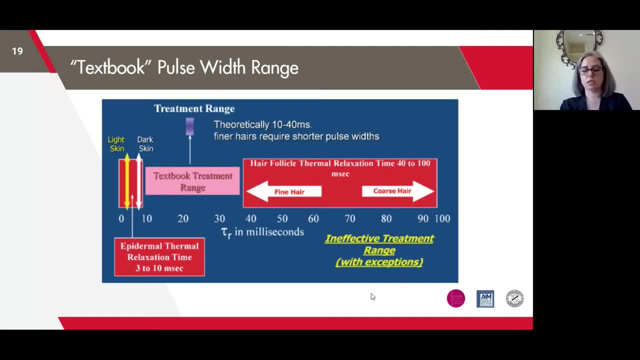 The range that it's recommended, as you can see in the textbook, the range of thermal relaxation, The range of presenting your device as pulse duration. The pulse duration, The range that you can do for hair removal, is between 10 to 40.. 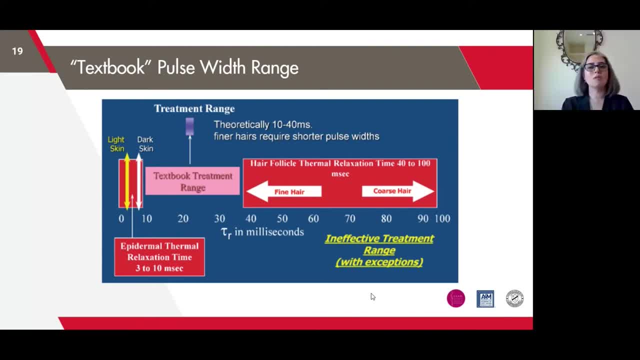 10 is above the skin, all the skin types. 40 is below all the hair. But it doesn't mean that any number between 10 to 40. For those of you who have experience, you will know that pulse duration of 10 represents a total different results than 12.. 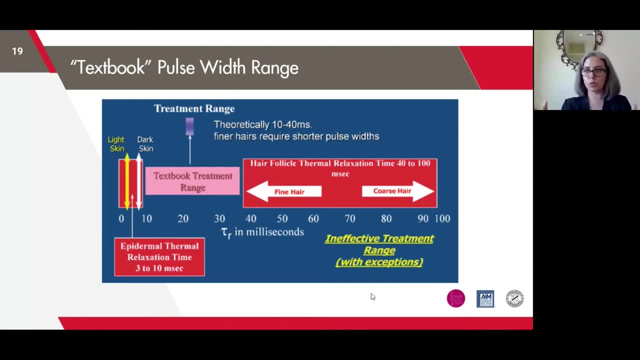 It's totally different than 15.. It's total different scenario than 20.. It's totally different than 30.. Adjusting the pulse duration Is your responsibility. I want you to know that with adjusting the pulse duration you can have magical effect. 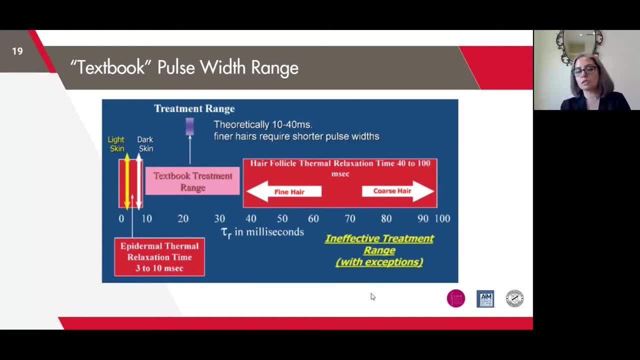 And you can have opposite effect of burning a patient like this with a short pulse duration. So pulse duration is an option in your device that puts your hand in so much of freedom. You can play so much with pulse duration, but only if your skin type allows you to do so. 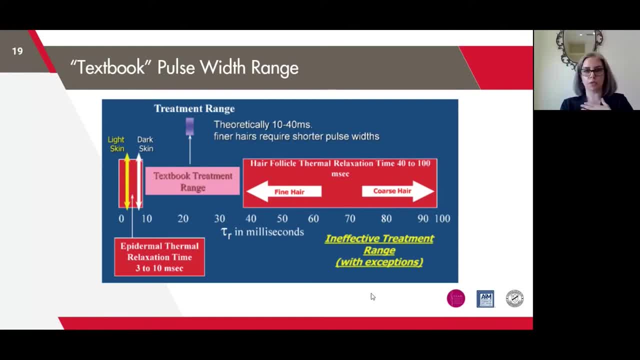 So, for example, if I'm skin type three, it makes a difference if it's my session number one or session number four In your session number. in my session number one, if I came to you with terminal hair, if you put a short pulse duration in my session number one, you burn. 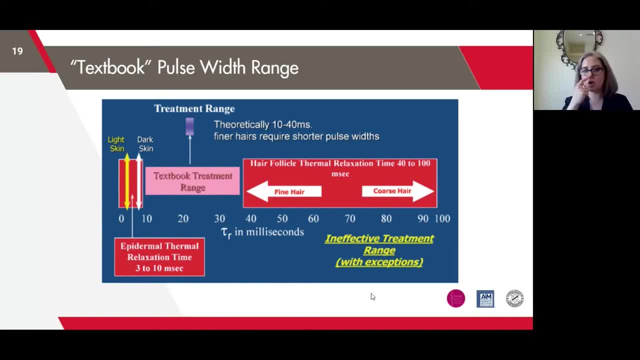 Although my skin can take it. for example, if you have the option of putting a pulse duration of 10,, 15,, 20,, 30. It's my session number one, all of them. my skin can take it. But if you put it at 10 or even 15 in my session number one, you will burn. 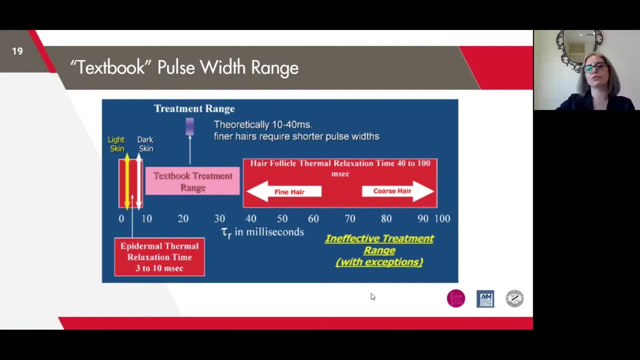 Why? Because you have so much difference, millisecond difference, between the number you have put and the number of my hair. If it's my session number one, my hair is thermal relaxation time And if it's black it will be between 80.. 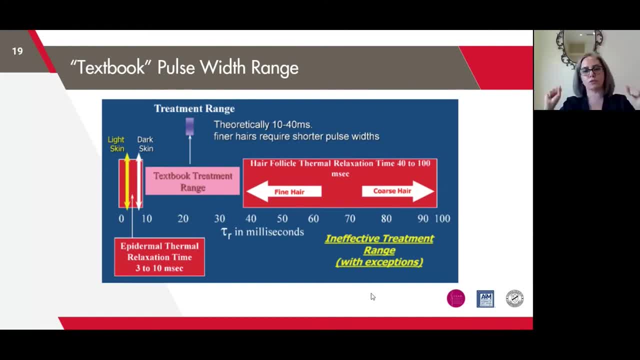 Now you put it at 10.. You have So much difference. You are too zappy, too short. in my session number four, Put it at 10.. Nothing will happen because at my session number four I my term or relaxation time of my hair is not 90 anymore. 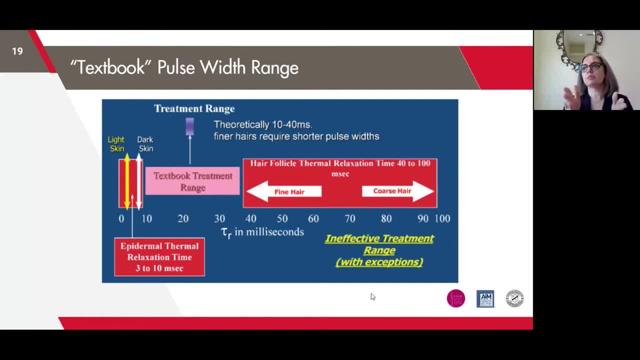 It's reached to 50, 60.. You made my hair not condense very light, not frequent, So now you can give them Stafely, but if you do give this 10 in previous session, you are Very. 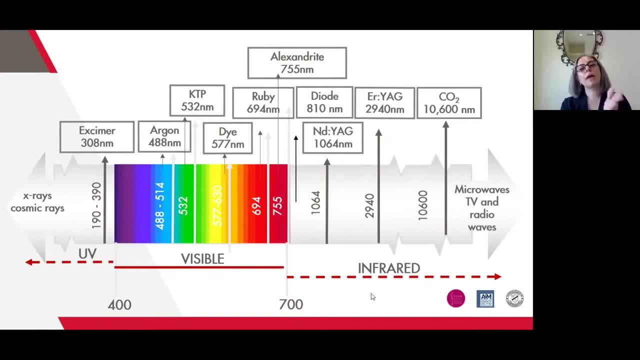 So these are some examples of famous devices in the market. We will just go to them together. Exciters are category of lasers that they are called as ultraviolet lasers. Exciters are lasers that are pure dermatological laser. They are ultraviolet. 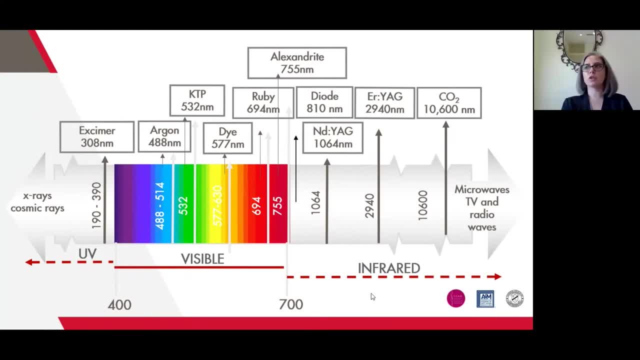 We have actually three. They are very short wavelengths, For example, excimer lasers 193, 3, 3, 3, 3, 15 nanometer, So very short wavelength. like excimer, I have to know that my laser doesn't penetrate deep inside my skin. 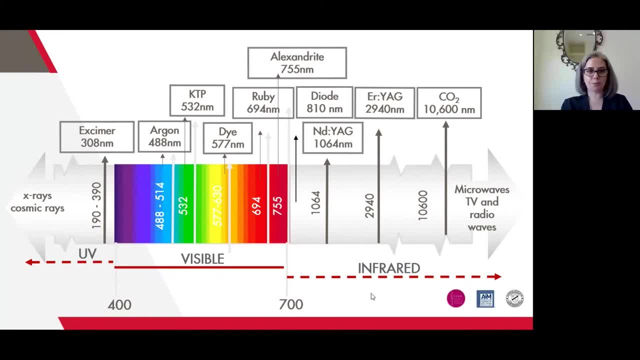 It stays out. That's why excimers are only used for dermatological lesions like psoriasis and vitiligo. That's why you are pure dermatologic lasers. Argon fluoride is the most famous Blue laser, with 488 nanometer. You know that we say blue is the best color for acne. 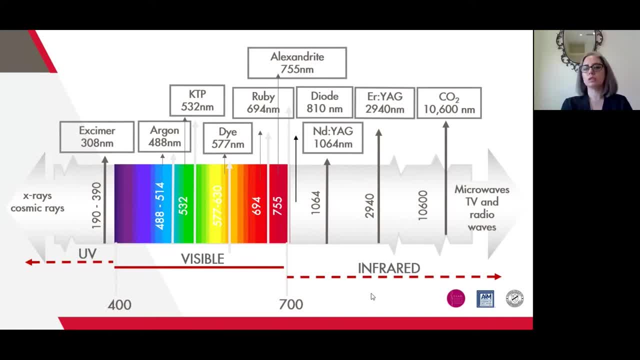 What you have to know. which skin type can I give blue? 1,, 2,, 3, that's it. We say green is the best color for superficial pigmentation, for epidermal pigmentation. Again, in who can I give it green? laser? 1,, 2,, 3.. 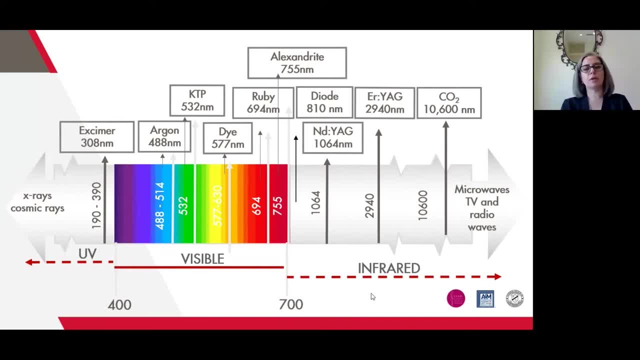 If I have a darker, deeper pigmentation or darker skin type, I have to use a longer wavelength like 1064, like MDR. We say yellow is the best color for superficial red vascular lesions. The two famous yellow lasers are pulse dye and copper bromide laser. 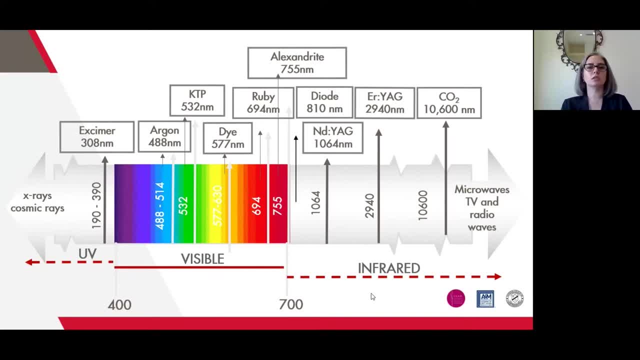 Again in who can I give a yellow laser skin type 1,, 2, 3.. If I have a deeper vascular lesion or my skin type is not one to do Again, I have to go and use India. Hair removal starts from Ruby, 694 nanometers. 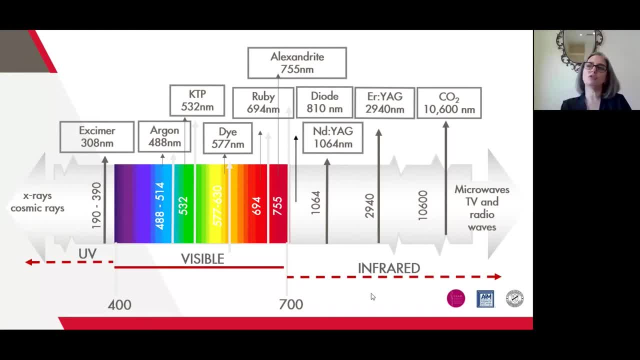 But you have to know that Ruby is a bit superficial for our hair levels In Eastern countries. in us usually our hair follicles goes to deep dermis. Ruby is a bit superficial. That's why you don't see much of Ruby in this region. 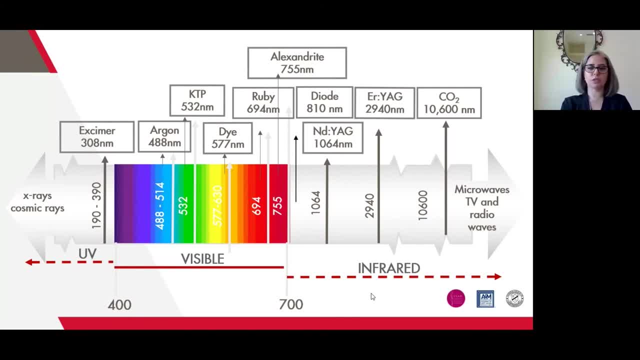 Plus, Ruby needs a really light skin to treat it. That's why The first wavelength that we do hair removal is Alexandra, and you'll know that Alex is considered, I guess, the most popular wavelength in herring. Now you know why. 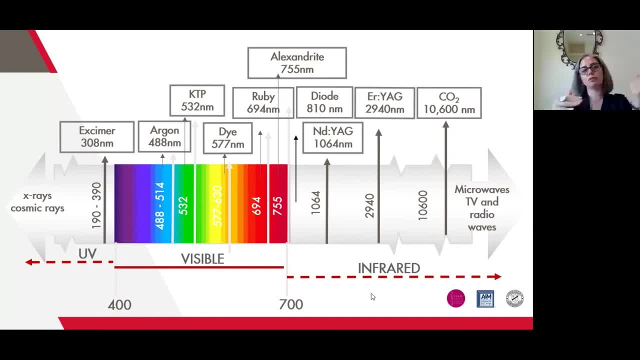 Because you know that Alexandra has more absorption curve comparing to others. shorter debate and higher absorption. The next wavelength for her one is diet. in majority of devices, Your diet for herring is a 10 nanometer. in some devices You will find 800. 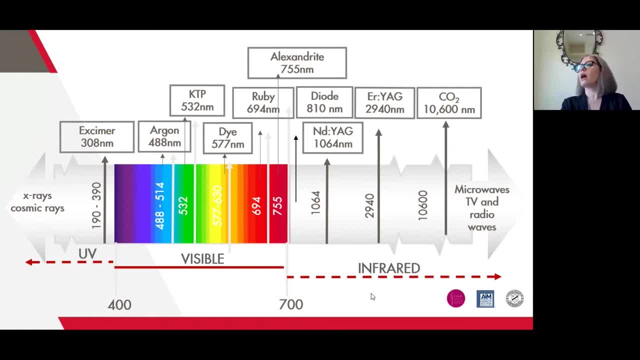 Your diet for herring, which we say. Alexandrite is used for skin type one, two, three, sometimes for guys. but you have to pay attention. if I use an Alex for skin type four, I have to adjust my parameters. Adjusting my parameters means what? 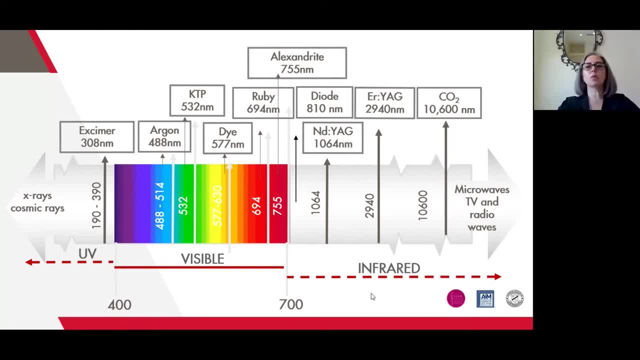 Reducing your fluence, increasing your post duration. You have to be safe on skin type four. Diet is preferred much more for skin type four And come Very little of five. skin type five, majority of five and six is advised to be treated with India for skin type six on the only India. and you know that with IPLs because sometimes we have IPLs in the market for herring. 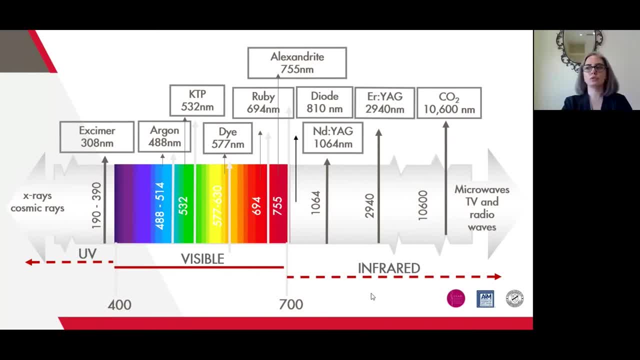 IPLs are mainly for skin type one, two, three, very rarely for not all the four, Very red. And then we have every on the app, which is two, nine, Four, Zero. And then we have CO2, which is ten thousand six hundred. again as a reminder, you remember, when I have water absorption, like in the peak of absorption, like I have very superficial penetration, 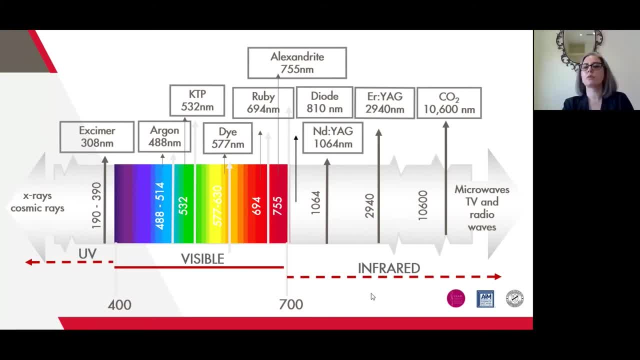 Airbnb. again, it's very superficial, like blue. it's 50 microns steps and CO2, it is not that much in the peak, but it's stealing the absorption curve of water, So CO2, I have 180 microns depth of evaporate. 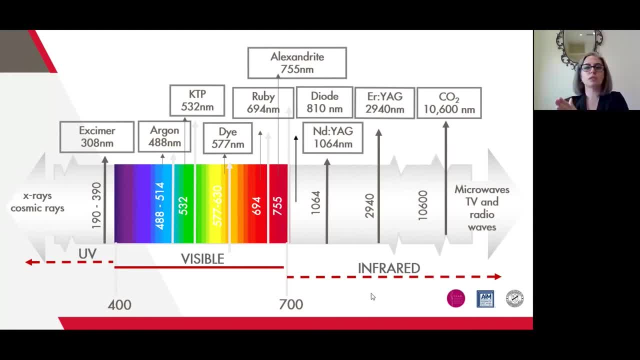 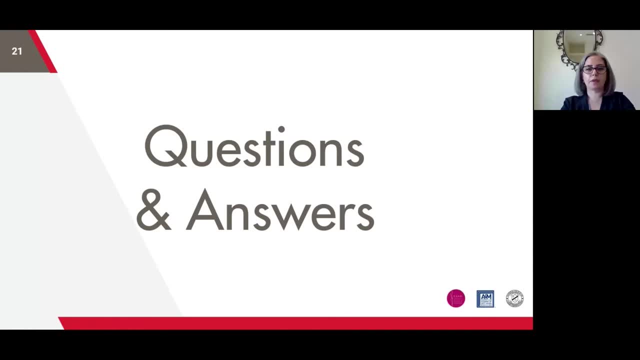 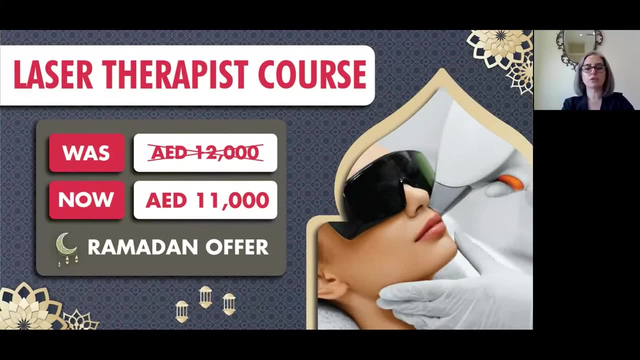 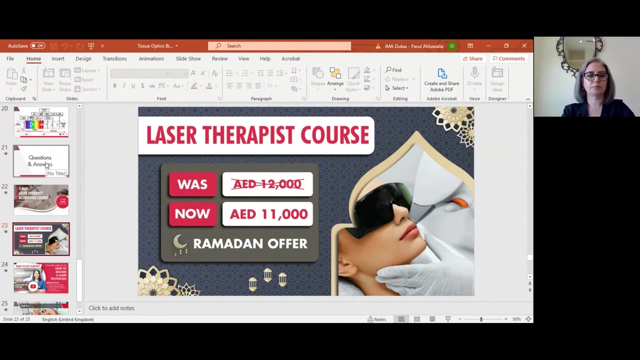 So, as you can see, in Airbnb, I can CO2, the laser van superficial, So I I want you to tell me if anybody has any questions. you can, you can get back to the questions And You can type any questions you have. 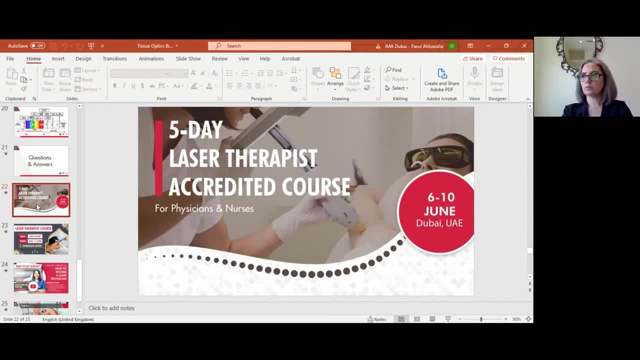 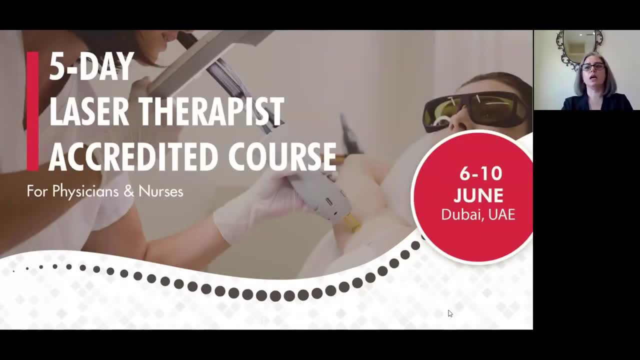 So, again, as a review, our laser course is a five days, a full five day course for those of you who want to do only herring, or once you can attend the first two days only. it consists of different lectures and for everything. 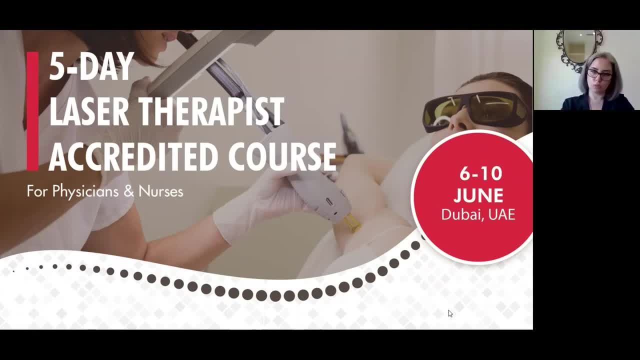 As I told you, we have the lecture and we have the actual models. So if you attend the first two days, you will get the certificate from NC NSC, which is the one of the most reliable certificate, and laser. in your certificate you will be laser technician or, if you attend the full weekly, laser therapists. 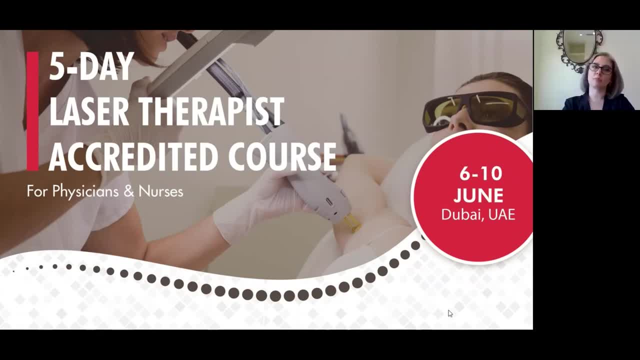 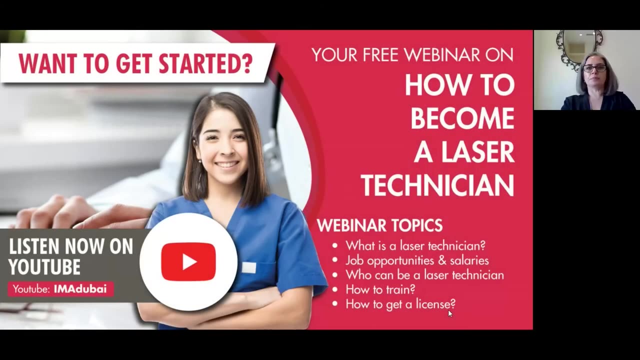 During the five day course, the full day course, we will talk about majority of technology, technologies available in Aesthetic. We basically talk about everything and we practice everything by with actual models and actual hands-on. So please let me know if anybody has a question. you can text me any question and I'm here to answer you. 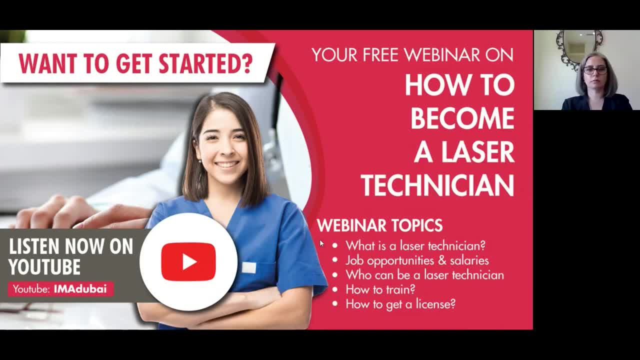 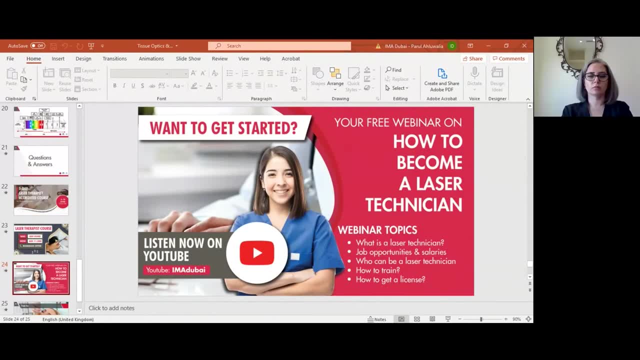 So the thickness. of course there is the direct relationship with pulse duration to the thickness of the head. Thicker the hair, longer the pulse duration, longer the thermal relaxation time. We said thermal relaxation time of the hair is between 40 to 100. 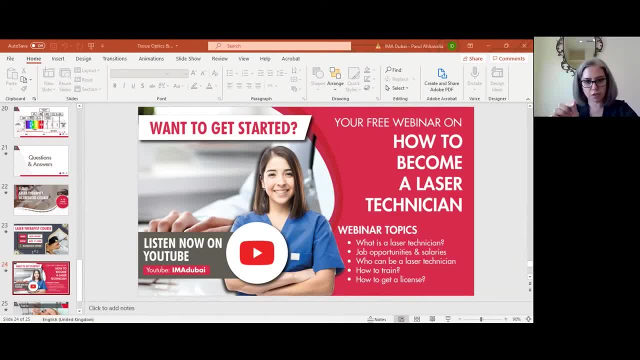 40 is for a hair that is a light pitchfoss hair. 100 is when your hair is thick and dark and black. So when you have a thick hair it means your thermal relaxation time is longer. Then I want to target it with pulse duration. 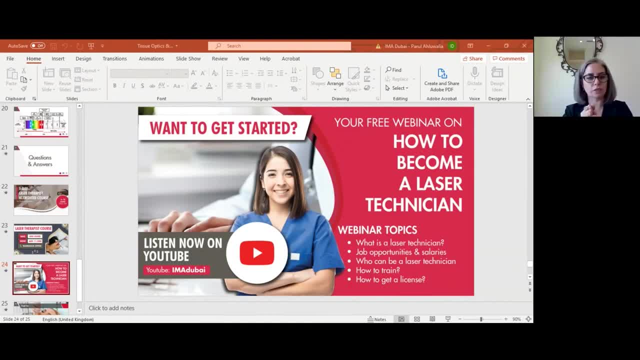 I have to consider this longer thermal relaxation time. That's why I gave you the example that if your patient is session number one, the hair is thick and dark. Don't approach the patient with a short pulse duration Now. your wide pulse duration is enough. 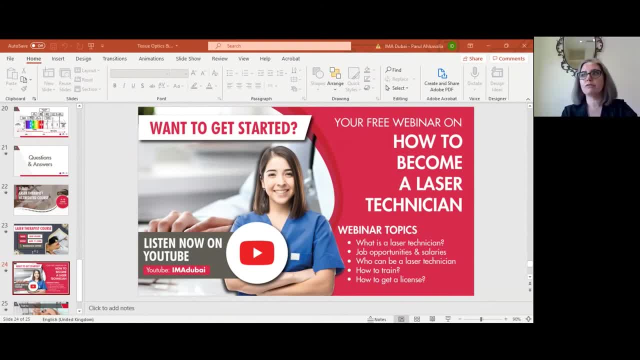 So thickness of the hair is very, very important. You have to know what is the color. how thick is the hair? The thicker has longer thermal relaxation time, So it needs a longer thermal relaxation time, Longer pulse duration. A thin hair- pitchfoss blonde thin hair- has a shorter thermal relaxation time. 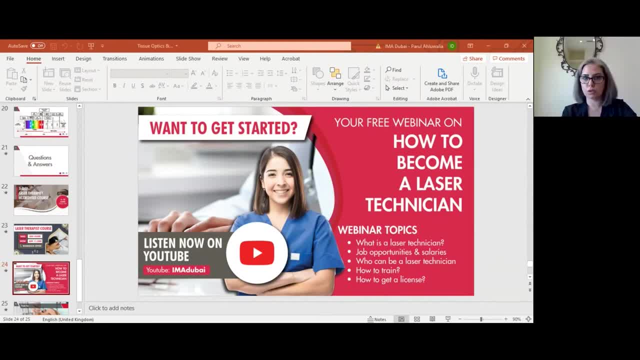 So in order to catch this hair, you have to target it with a shorter pulse duration. So thermal relaxation time. Somebody is asking what is thermal relaxation time? Thermal relaxation time is a time that 50% of the heat to anything is gone. 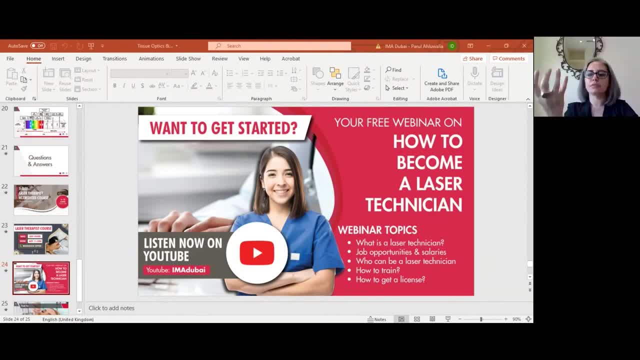 So when I heat her follicle then 50% of the heat is dissipated from this follicle. This time that half of the heat is dissipated is called thermal relaxation time And, as I told you, thermal relaxation time is dependent to the size of the structure. 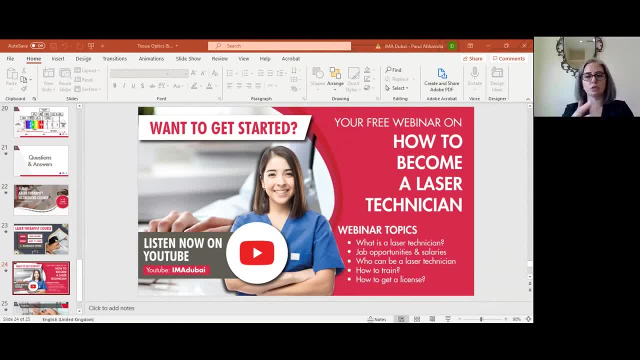 Smaller structures: they heat up faster, they lose the heat faster. Bigger structures: they heat up slower, they lose the heat slower. The thermal relaxation time of our epidermis is 3 to 10.. It means in me, who is a skin type 3, my thermal relaxation time of my epidermis is 3 milliseconds approximately. 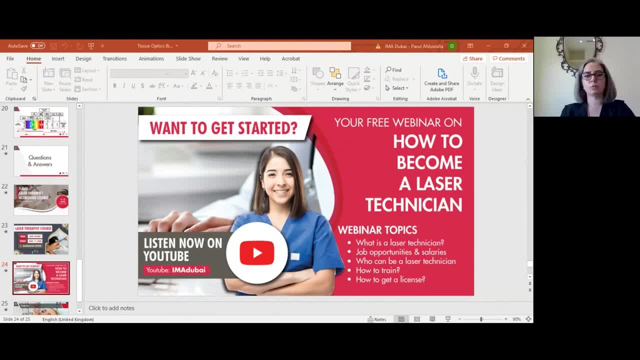 In a skin type 6, the thermal relaxation time is 10.. Sometimes in some textbooks you will find 0 to 10, because the skin type 1 can heat up in 0 milliseconds The hair follicle. then my hair is a light pitchfoss hair. 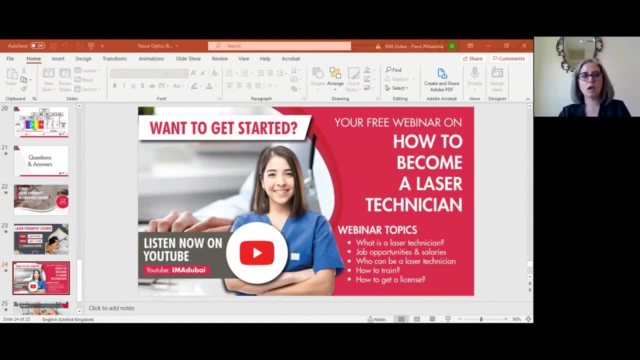 My thermal relaxation time is 40 milliseconds. For the terminal hair in scalp, bikini, armpits, men's beard, thermal relaxation time is 100.. LLLT stands for low level light therapy, or LEDs. LEDs are LLLTs, which now you know that they do rejuvenation. 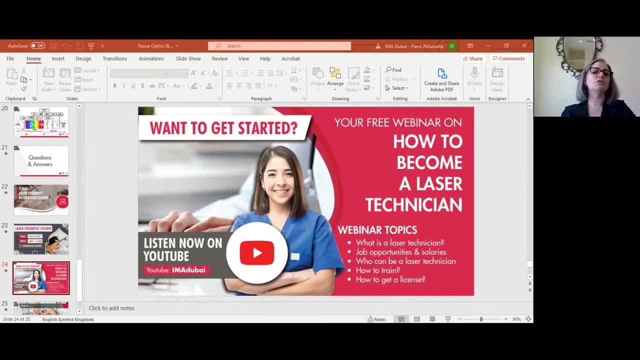 By photobiomodulation they stimulate mitochondria to give you more enzymes for metabolism. Blonde hair cannot be removed by the laser. So, guys, blonde hair, what I want you to know is not only blonde hair. One of the key concepts of a successful hair removal is: take a look at the hair at the back. 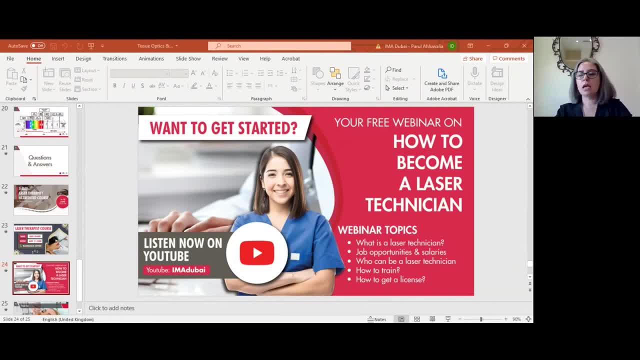 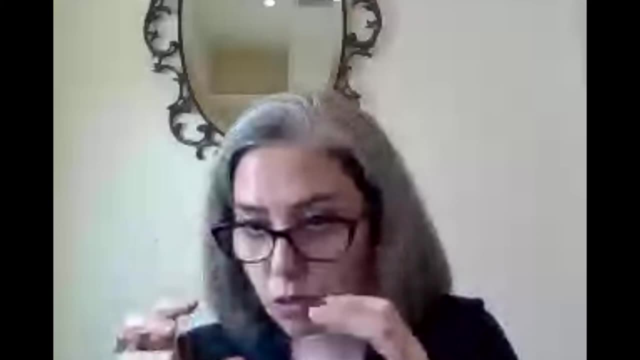 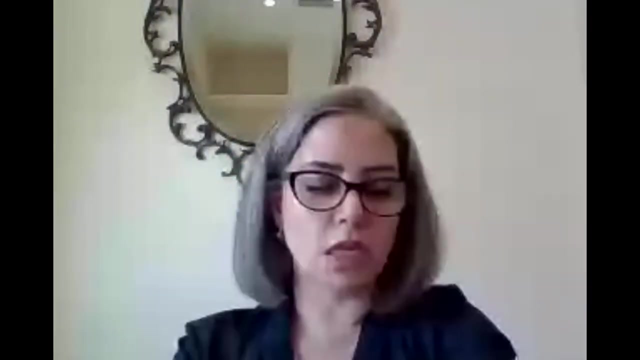 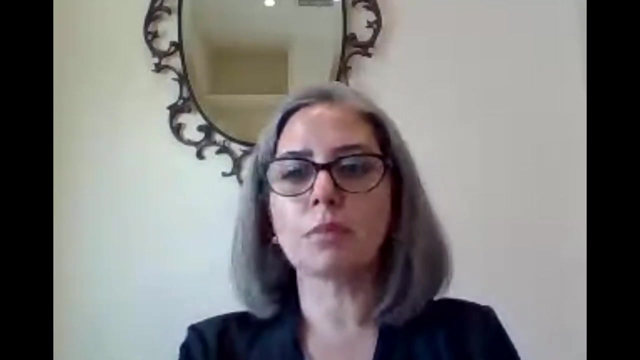 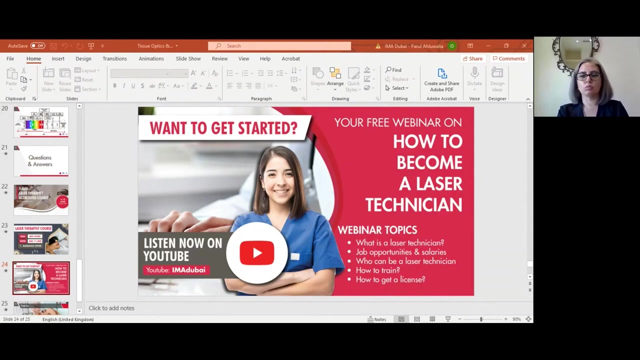 Take a look at the hair at the particular patient, Then you need a magnifier or glasses or you need to see the hair. So if I have a hair that is darker than my skin, then that hair and the darkness, the difference of the color between my hair and my skin, is totally visible. 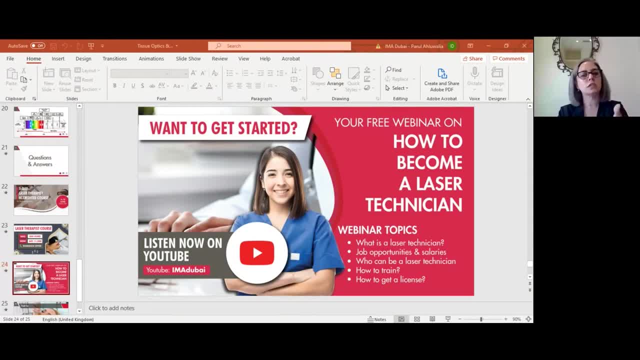 I don't need to put projector and magnifier, Then this hair will be removed easy. But if I have a blonde hair that doesn't have any color, Obviously this hair doesn't have any absorption. If I don't have any absorption, I don't have heat, I don't have healing. 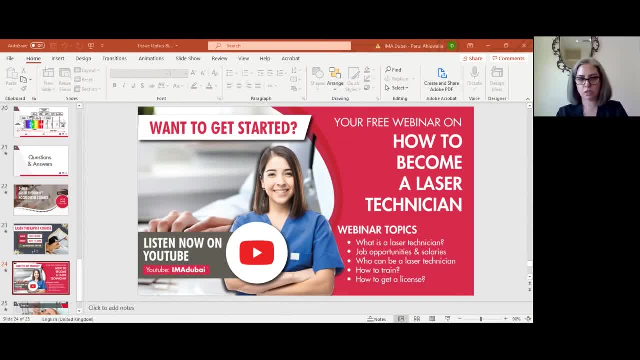 Definitely. white hair will not get any results. Blonde hair- if it's to the extent that this blonde hair is in a light person that makes the hair color similar to the skin color. No, you will not have effect with laser, But if the blonde hair has a bit of a color, 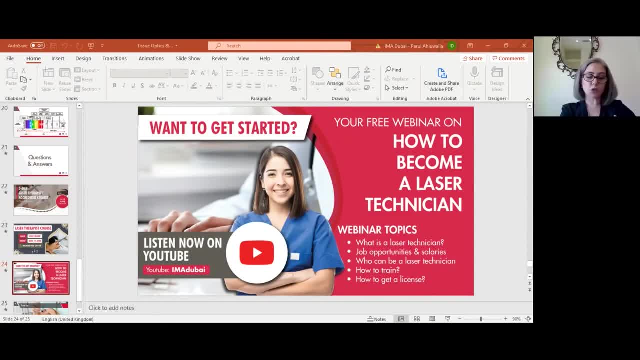 Then you can zap it with a shirt, Zap it with a short wavelength, with a short pulse duration, As you mentioned it yourself. So saggy skin for tightening. We have so many technologies for tightening. which is sagginess- It's not necessarily laser, guys. 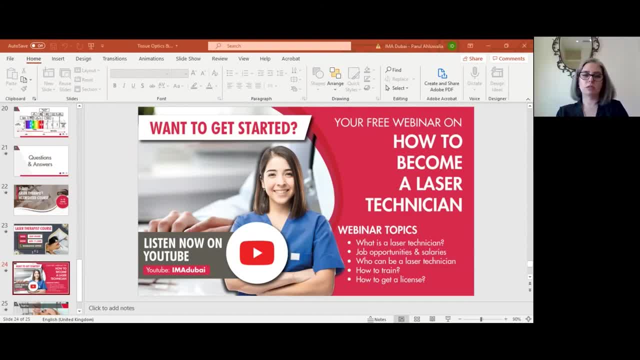 With laser. the treatment for tightening will be mainly resurfacing. With CO2 or radiofrequency, microplasma ablation or with erbium yak I will resurface the skin, especially with CO2.. And the result I get is tightening. 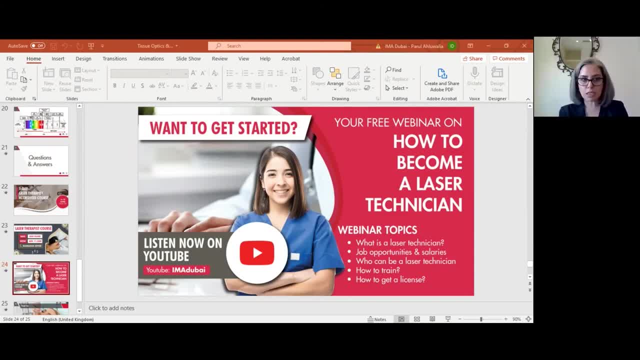 But we have other technologies that work with sagginess, which mainly is radiofrequency. With radiofrequency you go deep down the dermis, You stimulate fibroblasts And you are asking your fibroblasts to give you new collagen and elastin. 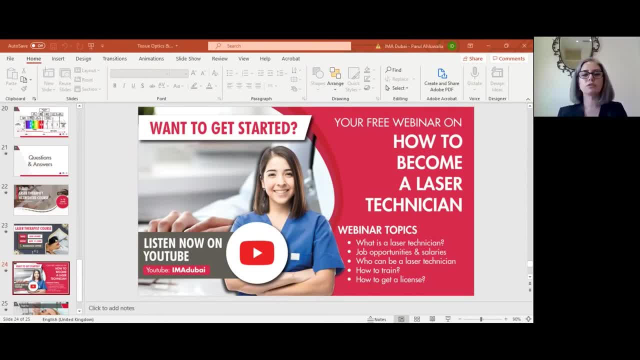 And we have very good results with sagginess, With radiofrequency, Depending different technologies. Radiofrequency comes in microneedling sometimes, But we have very good results with it. Not necessarily laser, But sometimes we have IPLs that they work. 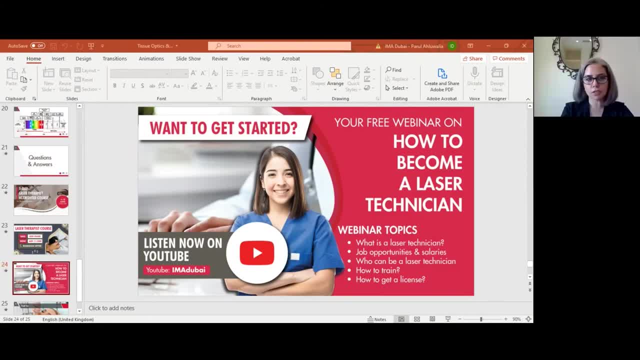 They mimic radiofrequency. They are called NIRs. NIRs as well. they are used so much for tightening. When do we get paradoxical hair growth? It's a very important question, guys. One of the first and basic measures Not to have paradoxical hair growth. 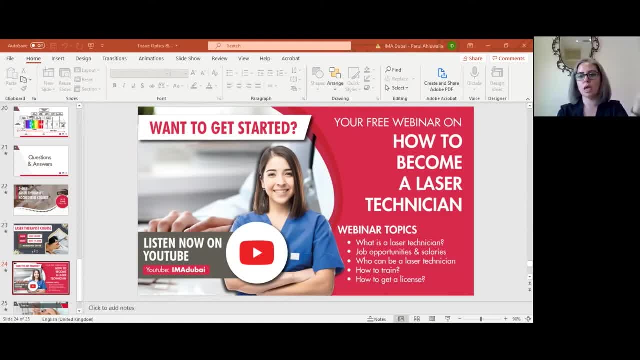 Is to pick your hair properly. That's what I told you. Ladies who don't have darker hair, Don't touch the area when there is no hair, Any area which is not appropriate for hair removal. When you touch it with laser, it's possible to have a paradoxical hair growth. 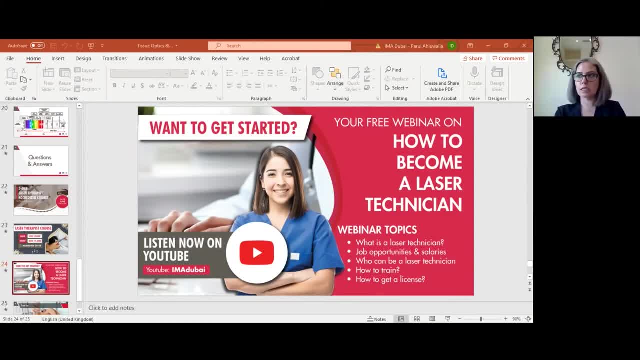 One of the problems happens in aesthetic clinics that they have full body hair removal Is that when the patient pays the money for a full body, She thinks- she or he thinks that the money is wasted if you don't touch all the parts of the body with laser. 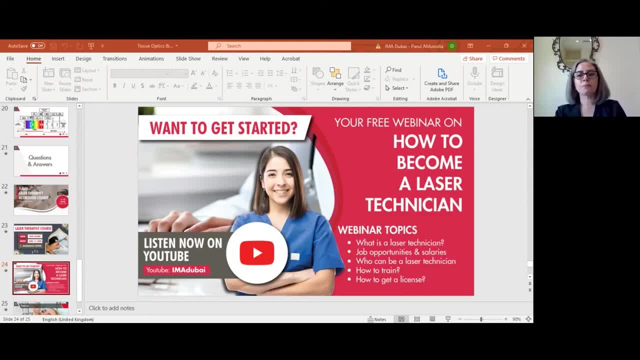 You have to sit and explain to the patient that if your hair is not appropriate for laser, It means it's a light color hair, It's a peach bus hair, It's a blonde hair. Majority of us ladies, we don't have a hair in our chest, in our abdomen, in our back that is appropriate for hair removal. 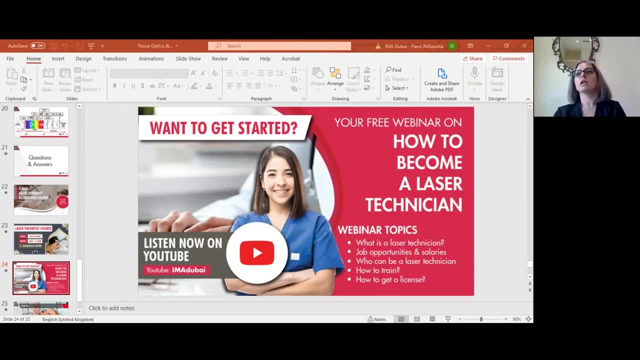 So if I come and touch it with laser and I give heat to it, especially if I have a slightest hormonal imbalance, I will have paradoxical hair growth. And please be aware of it, because paradoxical hair growth will kill you and the patient. 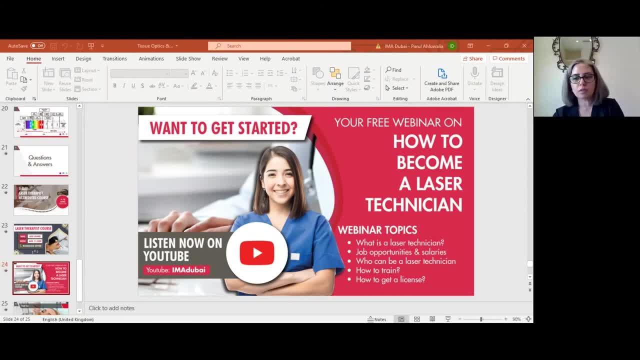 If she develops paradoxical hair growth then it's not a five to six sessions, She might come 10 to 15 sessions. So the first wise thing is not to hit a hair which is not appropriate for paradoxical hair growth. But there are two main paradoxical hair growths that it happens. 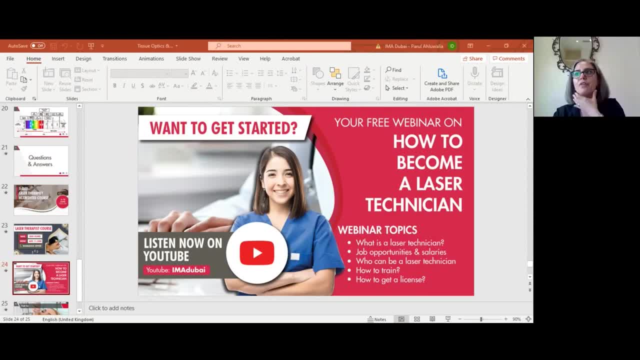 Usually in the face, Face of ladies. again, as my advice, guys try to avoid as long as as much as you can, unless this hair in the face is really a hair that it's appropriate for hair removal. And remember face of the lady is hormonal seat of the lady. 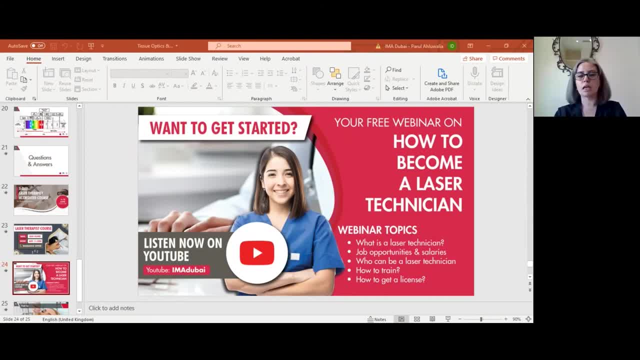 So any imbalance, Any hormonal problem will manifest its appearance here in the face. The paradoxical hair growth majority of the times comes with two groups. One in young girls that they develop dark hair. here They never had darker hair Once they started touching their face with laser. they develop darker hair. 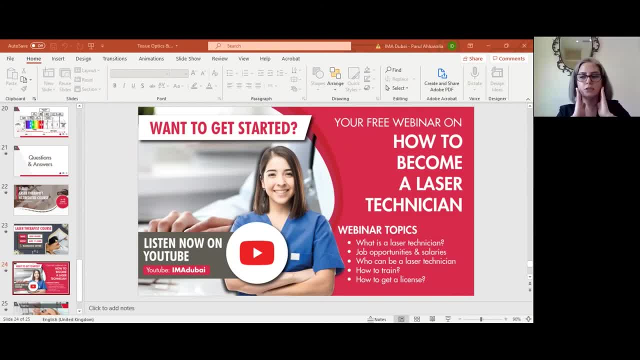 The reason is the heat of a scattering which goes to surrounding tissue is not enough to kill, It's enough to stimulate. So If you had a young girl coming to you to do this part, only during the treatment time, all the time during the treatment, keep two ice packs here to avoid any heat going to the jawline. 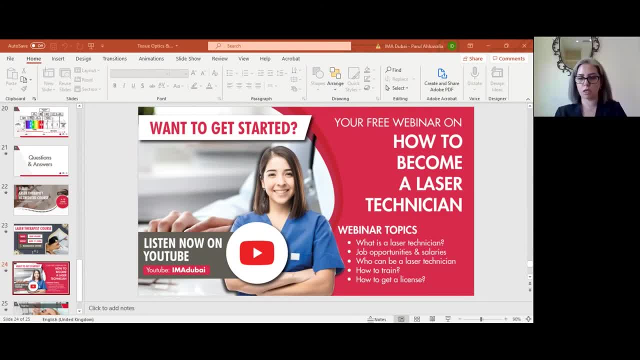 This is how to avoid paradoxical hair growth in young girls, And a harder paradoxical hair growth happens in pre-monopausal and monopausal ladies. When they come after one or two sessions, they will tell you that you turned all my hair. 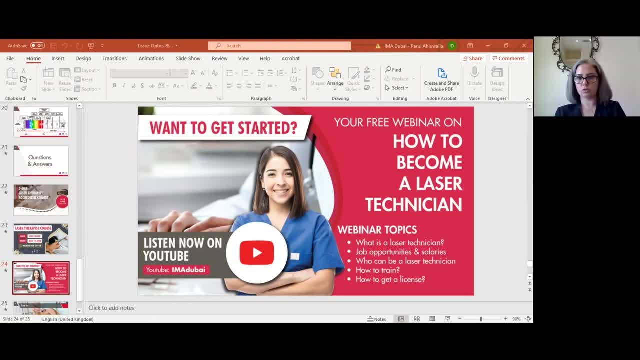 You turned all my hair here to white, Which is true. We turned it to white. First of all, your advice to the patient is: never wait until your hair turns to white at that age, Because then white hair of course doesn't respond. 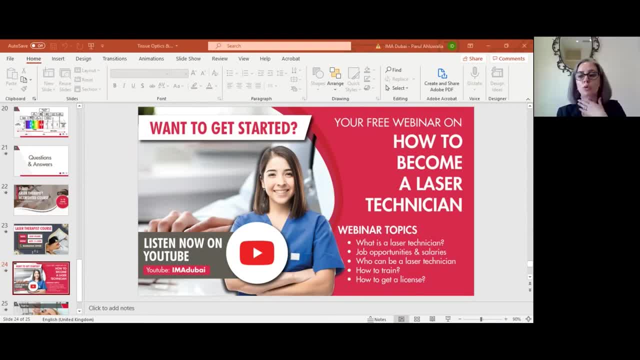 And, as I told you, since my face is the hormone seat at the age of monopause, my body is waiting for any switch to turn, to switch to white At that age. Sometimes, those of you who don't want to give pain to the patients 50, 60 year old, or they are sensitive to pain or for whatever reason, 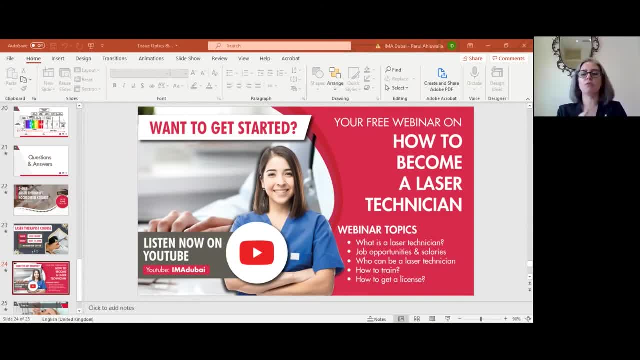 If I am not sure of what pulse duration and what fluence to give If I don't remove the hair completely. Basically, what I mean is if I cannot give a 70 degree hair temperature to the hair. here I give 60 instead of 70.. 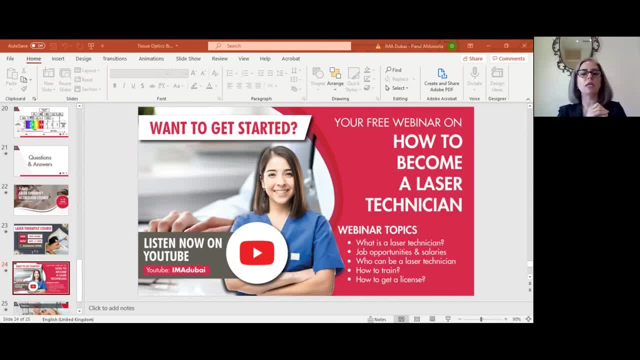 What happens is that I partially remove the melanin in this part And for my body it recognizes as it's a time for me to turn to white And it shifts. all the hair shifts to white And once it's white, only electrolysis is your solution. 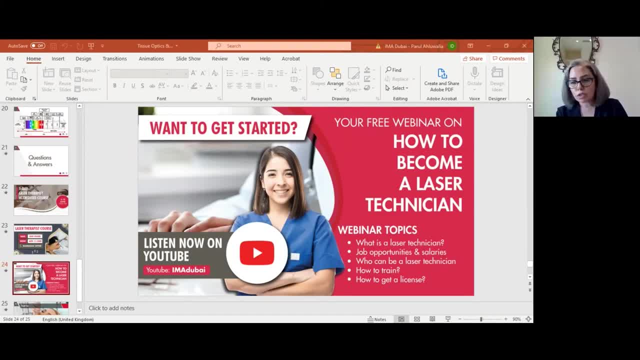 Then you cannot do anything else. So how to avoid this paradoxical hair growth When you have a monopausal lady? try to find the highest fluence that doesn't burn the patient. Do a patch test, Find your high fluence. 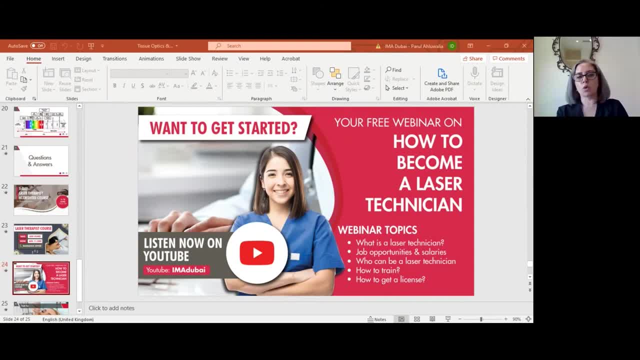 So we use the short term HLA And this is the były. We will show you all the three things that we use. This is a combination of the. So soft light doesn't help in hair removal Guys- soft light. 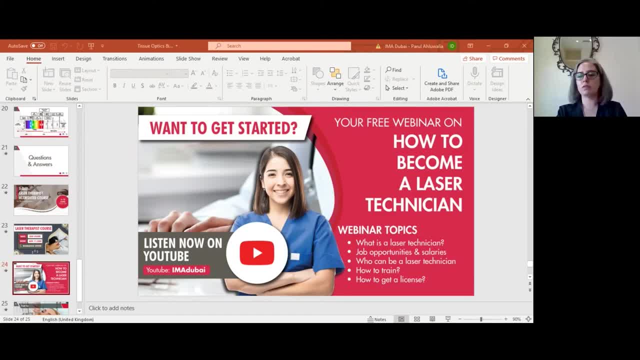 They only lighten the hair. They don't do hair removal. For so many patients they really don't need to do hair removal. as I told you, So many of us ladies, our hair is already peach, bust, So the hair- or doing a soft light. but of course so many experienced after several 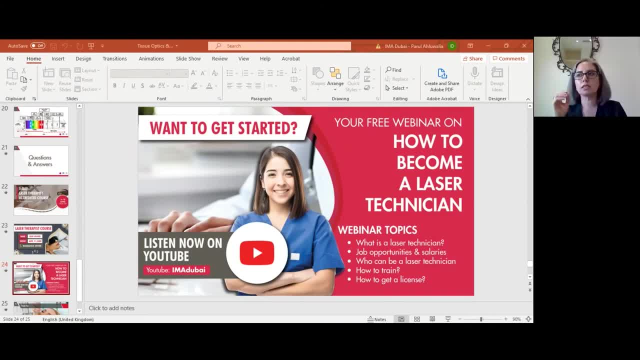 sessions of soft light. the hair starts getting weaker and falls off after. but this is not a hair removal. you know that. a laser hair removal- you will give 70 degree and you kill the hair. soft light doesn't mean that you switch. laser just shatters, removes the pigment from the hair temporarily and your hair grows in. 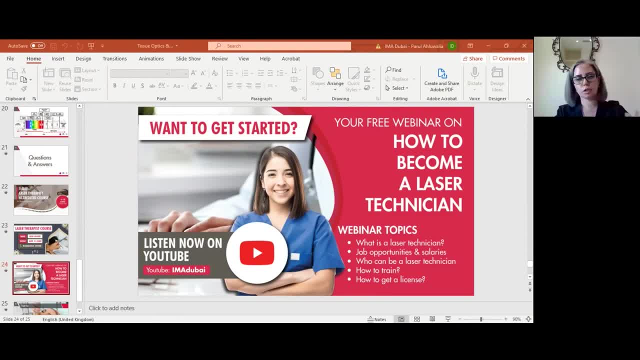 a longer pace in a longer time. lighter color you. so if you follow IMA, you will know the dates of the five days course. if you want, I can explain to you. in our day one we have different lectures about the main lectures, the topics that you will have in your exam. day two is mainly the 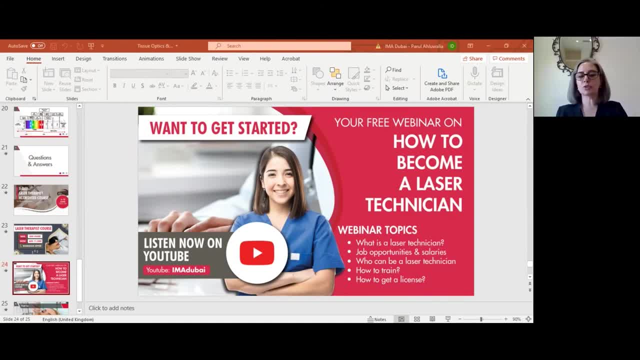 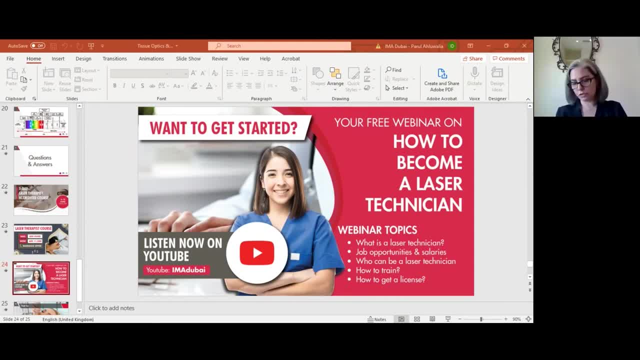 we are doing resurfacing. you see, all the three resurfacing, obviously for every day. we have lectures in the morning, we have hands-on of what we talked about in the afternoon, everything we talked about practice. so we will have the lectures of resurfacing and 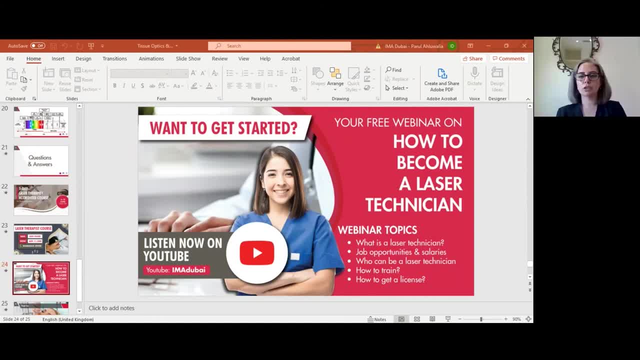 fractional treatments. in the afternoon we will actually do an erbium yacht, co2 and our plasma micro needling, our plasma resurfacing. and the last day of the laser course is the day of contouring, which we talk about all the technologies available for contouring, for tightening, for reaching to. 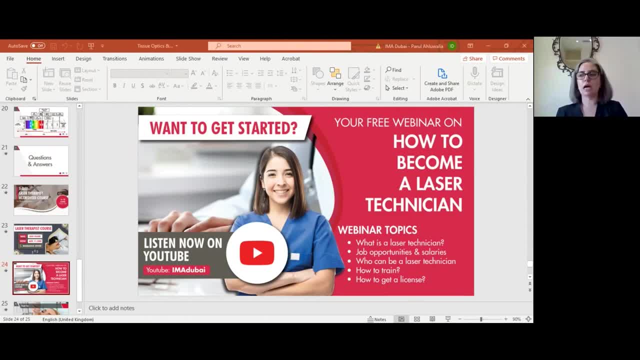 facts and in the afternoon, of course, we have the hands-on and the participants will have the exam afterwards. you have to attend the online first. you have to finish the online module. the online module consists of different modules that you will finish it after filling the online module. you 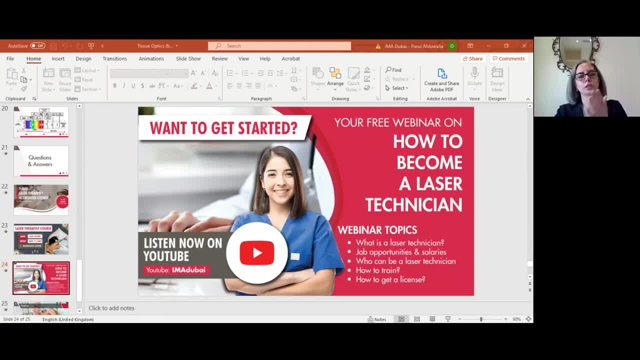 will have an email from NCLC and then you will be eligible to sit for the actual exam after finishing the actual exam, which usually is hundred questions, multiple choice, three hours exam. hopefully, if you pass the exam, which needs a 70 score to pass the exam- 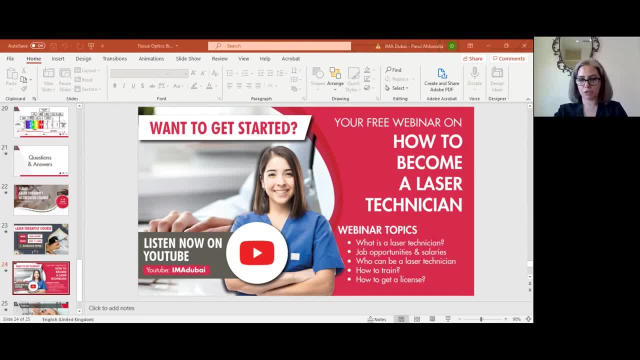 you will be obtained with NCLC certification. please google this certification. I'm sure that you all know that is one of the most reliable certificates. Our place that we are talking about IMA Dubai. I will want you to follow our website of IMA Dubai. 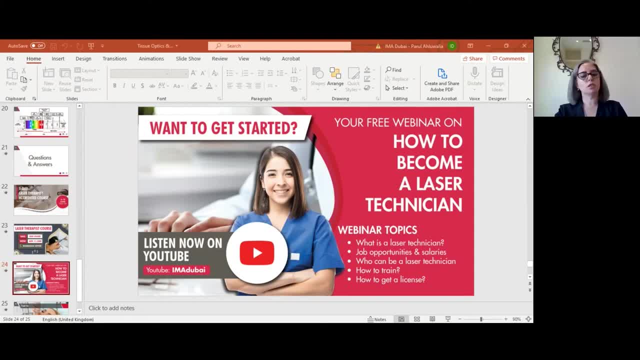 Dubai and then you will get much more information if you visit our website. and those hair. darker skin: yes, her removal we can do in darker skin, but we have to pick a longer vase like NDF. We can do NDF for dark skin tones And nowadays we have different technologies. 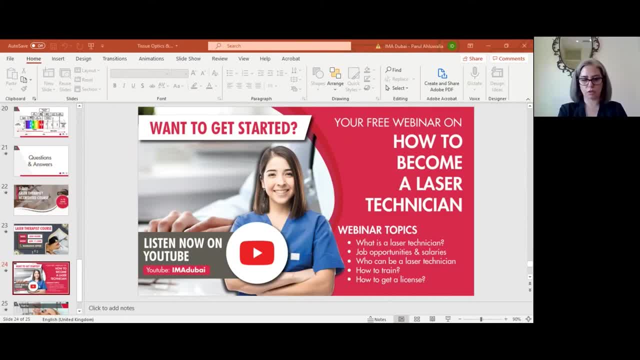 that it's motion technology that we can do for darker skin tones. What I want you to remember is that every device is different. I don't want you to get yourself confused with the numbers that you see on devices. In one device, your fluence. 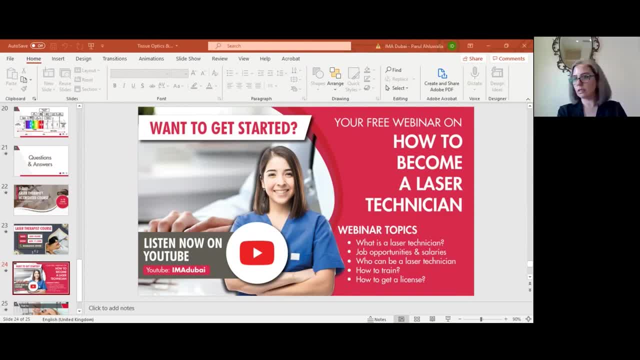 10 is a high fluence. In another device, high fluence is a 60. Be sure that in any clinic you are working, you have to get trained with the devices that you are working with And you have to work with the manual of the device. My advice is, with every device you see, work. 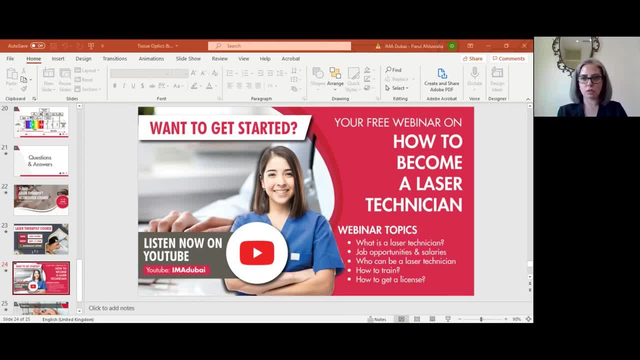 with the manual of the. going back to the protocols and manuals of the devices, It takes you one or two or three patients to get used to the manuals and numbers of the devices. What I want you to pay attention is the concepts short pulse duration or long pulse duration. 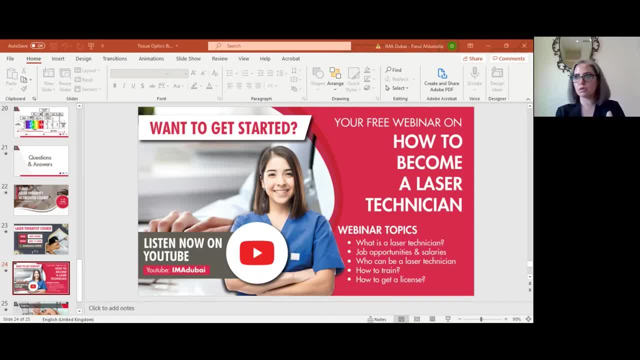 high fluence or short fluence, small spot size or big spot size. This is more important than the numbers that you are talking about. So, with the question that somebody asked about the short pulse duration of 20 and the fluence of eight or nine depends on which. 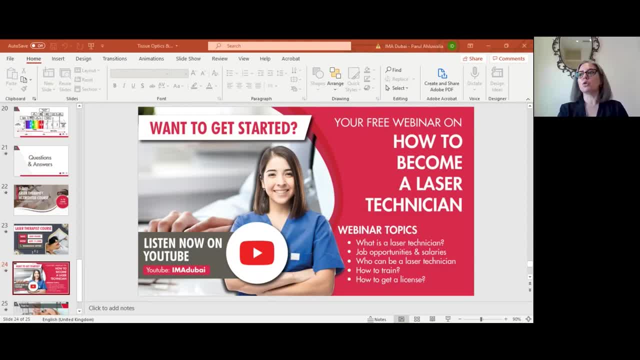 device you are talking about. In general, when we are talking about Alex, we are talking about skin type one to three. We are not talking about darker skin types. So parameters of Q-switch laser for NIVA sub-Auto can be different depending on the device. 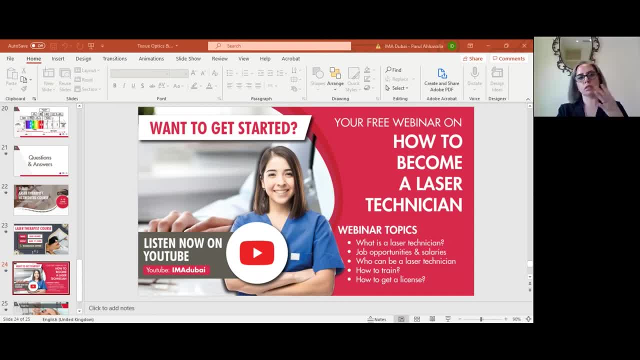 As I told you, in my device my Q-switch laser can be in one parameter. in another device it can be in another parameter. Go back to the protocol of your device and check what is the recommendation. Guys, be sure that every device has a protocol, something like a booklet that all the indications that 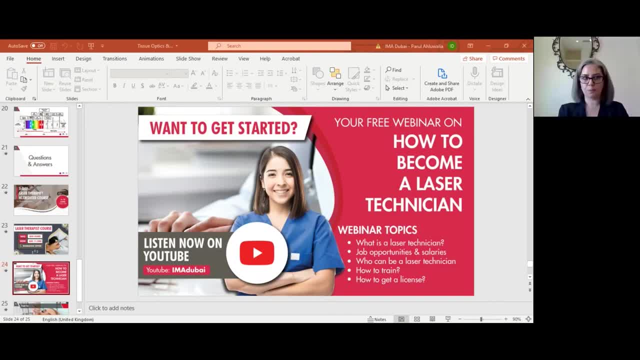 you can do with it. it's written in the booklet, So please go back to it, read your booklets and have access to it. If you don't have it in your clinics, ask the provider to give you the booklets, because this is very, very important. 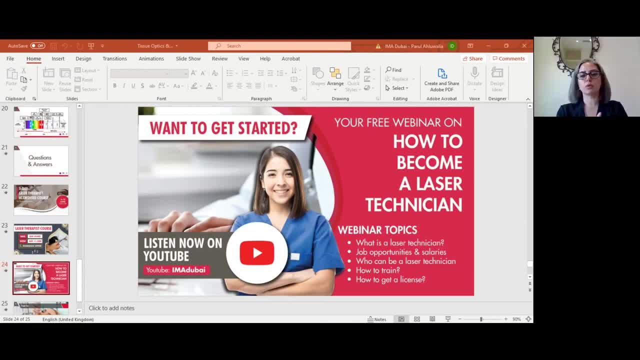 Fluence is not only set based on the protocol of the book. Fluence is set based on patient sensation. The protocol is telling me do with fluence 25.. When I zap the patient with 25, she jumps. She says I feel like eight. I have to decrease the fluence according to. 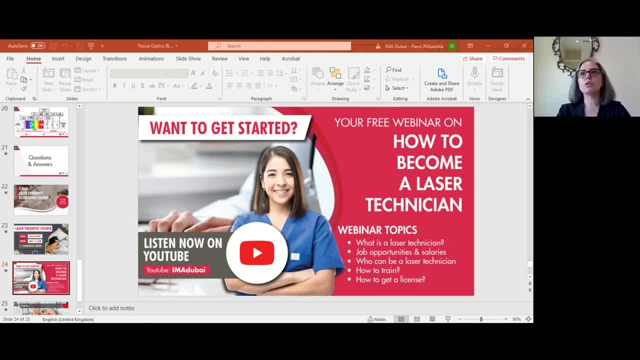 patient sensation. The protocols are just rough guidelines for you, but they are very, very helpful. Any more questions? This is a very hard question. No, Unfortunately I don't have a personal favorite device among all the devices. You know that every day we are talking about biggest market, I guess. 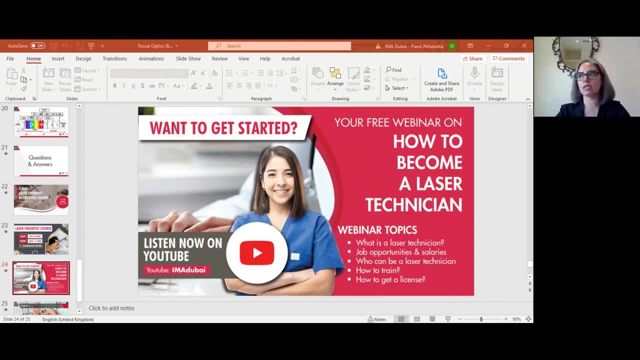 in the world. Every day you will see new devices, upgraded version, new models. What I want you to know is that you have to know the concept, You have to know the technology And then you can go back and see what this machine can do to you. 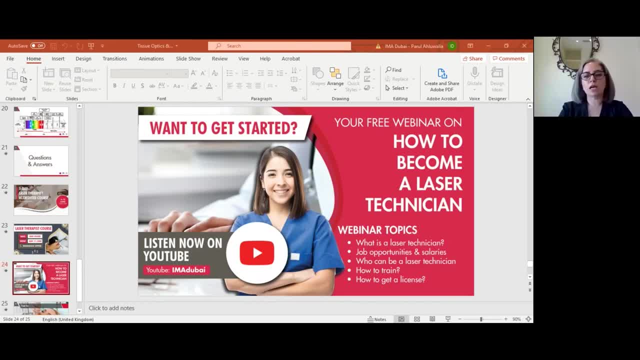 In Candela. okay, All the concepts that we are talking about in those of you who are working with Candela is a bit different. Why? Because Candela is a device that uses a fixed pulse duration, which is usually very, very short. That's why it's so important to know 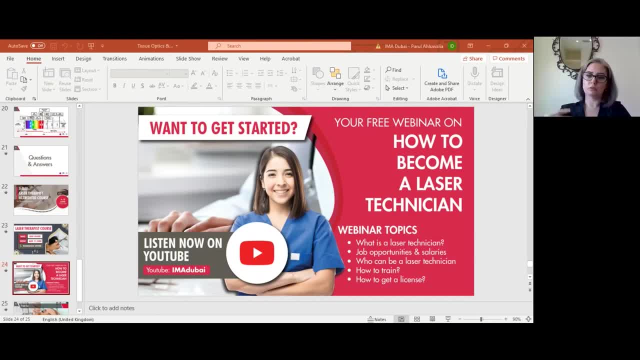 that it has the most aggressive cooling, which is cryogen. In Candela and the first devices, if you remember, the pulse duration was fixed on three milliseconds. So what happens is that with the three milliseconds, if I don't have a cooling, I basically burn everybody's. 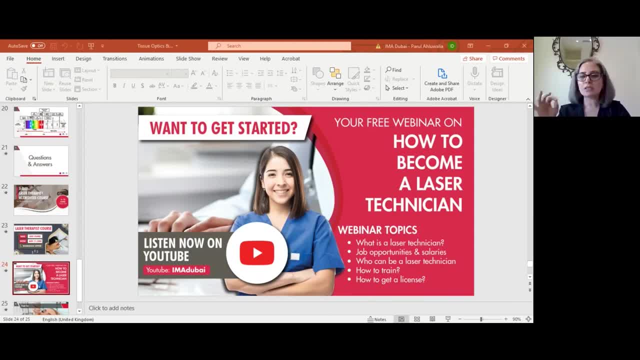 skin. That's why the most effective cooling technique is considered to be cryogen. Forget about the fact that cryogen is a very aggressive, very strong, but very, very, very good, very effective cooling, but very, very good, very effective, very, very effective turns You. 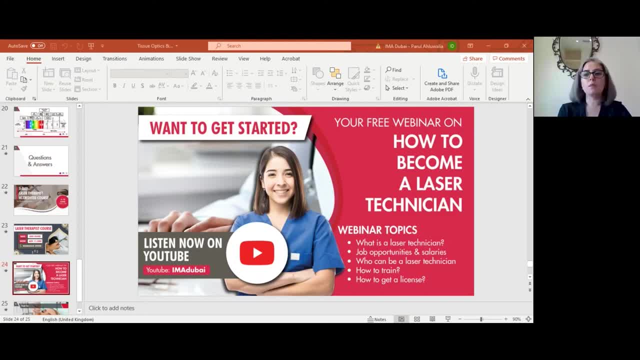 aggressive cooling guys, cryogen by the company that makes it. they say if you hold the cryogen more than 80 milliseconds it guarantees a freeze burn. we have so it tells you. first thing is you have to be careful with cryogen. don't hold the cryogen without a laser. we have so many patients that they get. 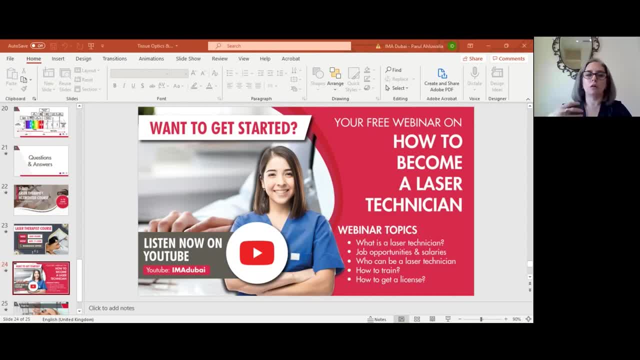 pigmentation just because of cryogen, considering that I have a very, very short pulse duration here. so with Candela my setting is a very aggressive setting. the company tried to compensate this aggressive setting with a cryogen which in the market you will find so many patients, as I told you, it has initially. 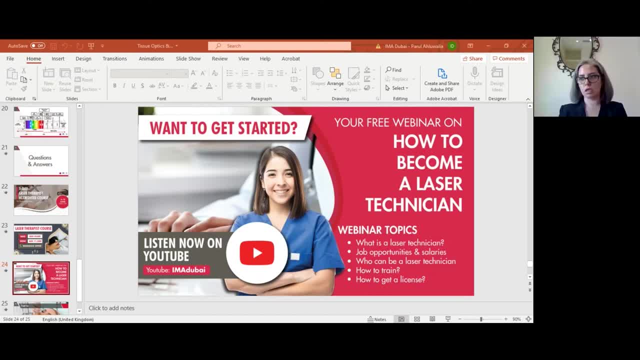 from the first session. very good results in terms of her removal, but very big risks. a dark patient, a skin type 4, so many they get pigmentation. The best heating method? I cannot tell you the best, because the most effective is cryogen but it's not the best because it has so much problems with pigmentation later. 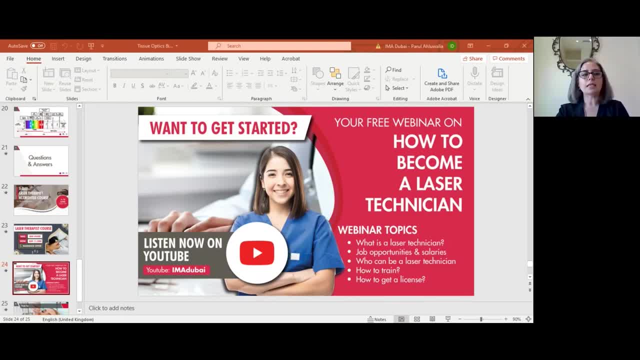 because it's a very tricky cooling technique. The best nowadays is considered the devices that they have the contact. the sapphire cooling is considered nondectin, long 영양. cassette and acrylate. Two are frequently usedya have the contact. the sapphire cooling is considered the devices that they have the contact. the saffire you're cooling is considered. 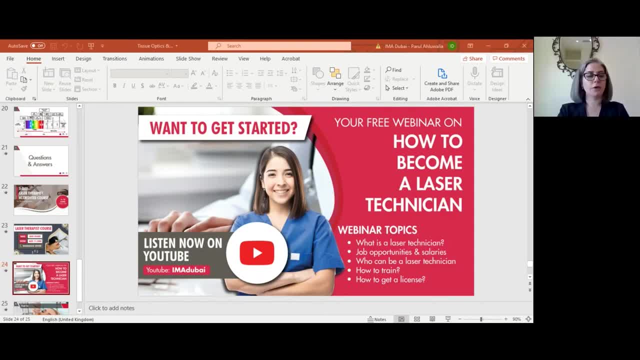 they're the best, better cooling than cryogen. You're welcome, my dear. So give me more questions. whoever wants, No problem, you're welcome. Thank you very much. Usually our participants, of course, are doctors. 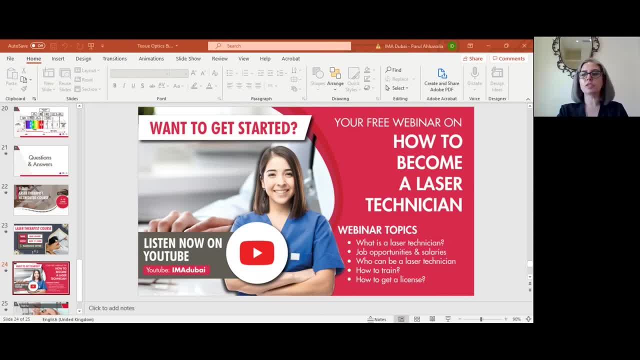 dermatologists, plastic surgeons, GPs, nurses, beauty therapists. Look, the matter is that for participating in our laser course we don't have any limitation. Limitation comes whether you actually can work with these certificates in Dubai, for example. 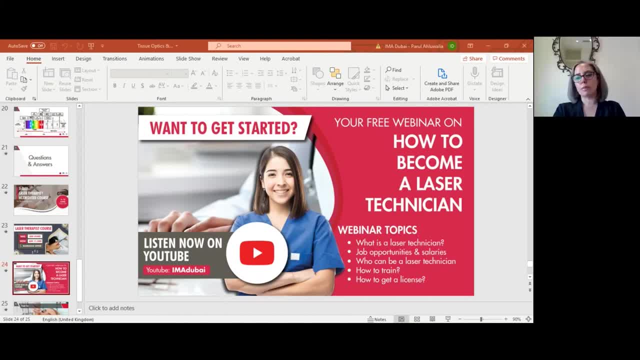 or not. According to DHA, you have to have a medical background. definitely beauty therapists they can, nurses they can. So we have sometimes dentists and other professions. Even if you are a housewife, you can participate. 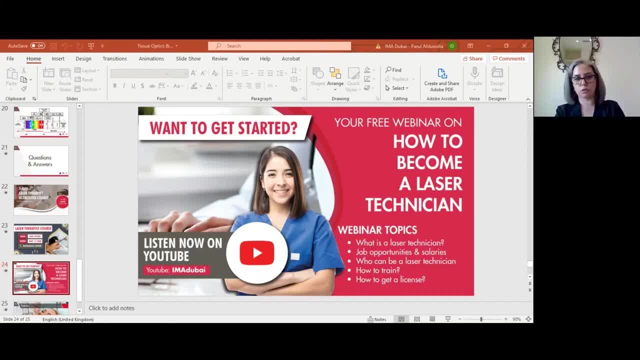 in our course, but then you cannot practice with it according to the rules and regulations. So it depends on the rules and regulations of where you work with. It makes a difference, but usually in order to be able to practice you have to be in a medical background. 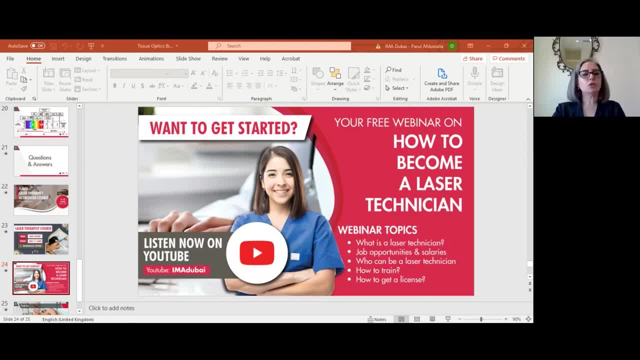 Somebody asked which one is better: Q-switch or nano. Q-switch or nanosecond, it's the same guys. Q-switch lasers- their pulse duration is in nanoseconds. If you meant Q-switch or picoseconds, picosecond lasers. 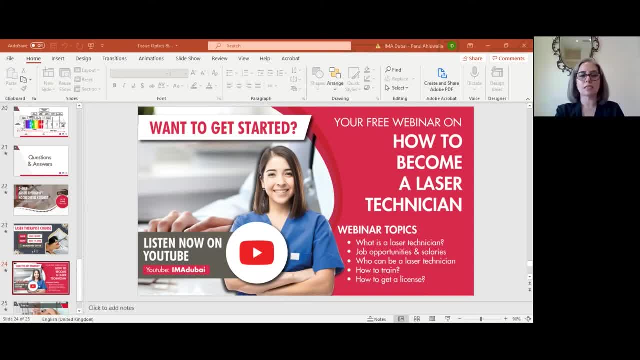 they are shorter in pulse duration so they have even less speed compared to nanoseconds. So active medium: somebody asked what is the active medium of diode laser. It's diode Guys. the name of lasers are referred to. name: 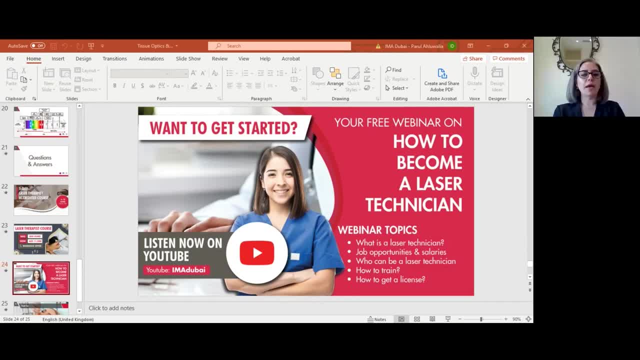 of the active medium of lasers. So, depending on, depending on the active medium, depending on the material that I have in the active medium, my laser is different. In CO2 laser In diode, my active medium is a CO2 gas. 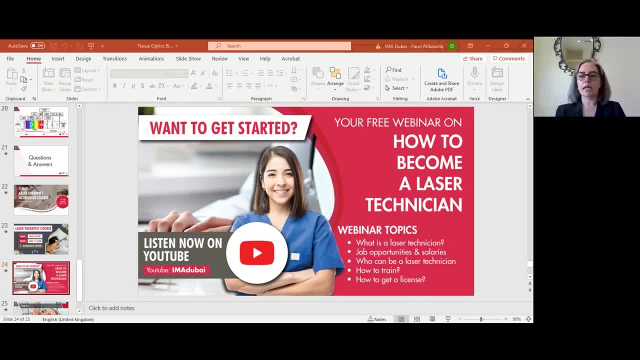 In ruby alexandrite, a endiac, my active medium is a crystal, is a solid crystal. In pulse dye laser, my active medium is a color that I added to alcohol, is a dye that I added to alcohol, so now my active medium is a liquid. 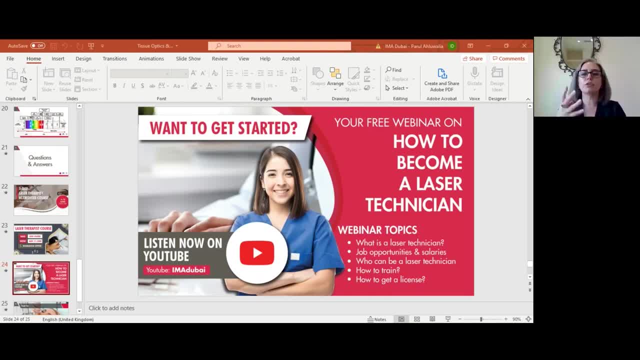 In diode. diode is considered the fourth matter. So we have solid liquid gas, which we talked about. Diode is considered the fourth matter. Diodes are considered semiconductors. Semiconductors, you have to consider them like broken glass. 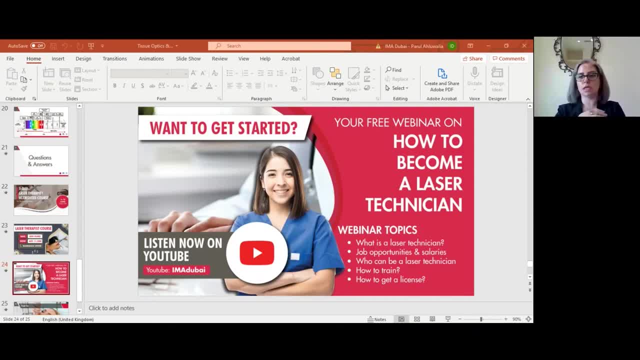 Diodes are tunable mediums. It means because there are smaller particles of solids, you can get any wavelength you want from diodes. You means not us engineers who make the laser In general, for a laser medium is none of my business. 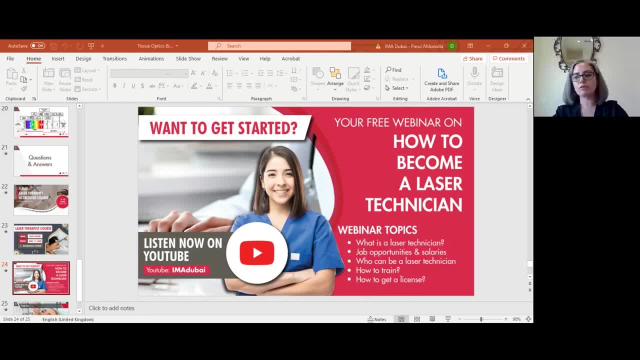 in practice. What matters for me is what I do. What is the wavelength coming out of this medium? In diode lasers, the medium is diode, which is like a broken glass. It's called semiconductor. So my diode that I work with hair removal gives me 810,. 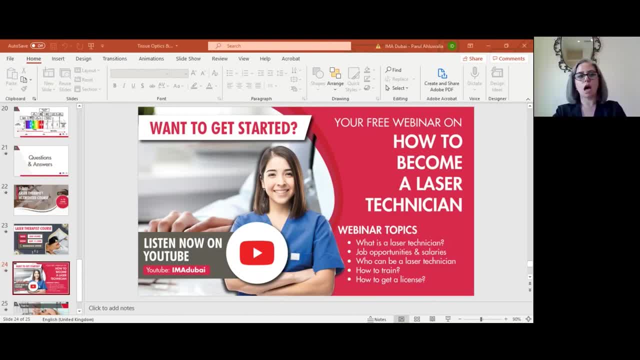 but I have diodes that are 550.. I have diodes for liposuction- 930.. I have diodes for rejuvenation that are 1400, because now you know that diode is a smaller particle. I can get any wavelength from a diode that I want. 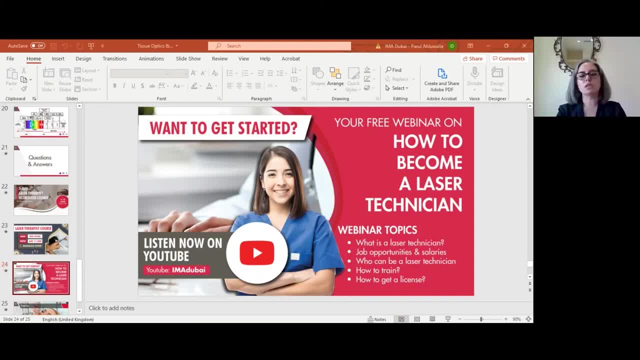 What matters for you is what is the wavelength that you are getting? Yes, picosecond definitely is faster than nanosecond, so it has less heat comparing to nanosecond. That's why so many there are now in the fun of doing.